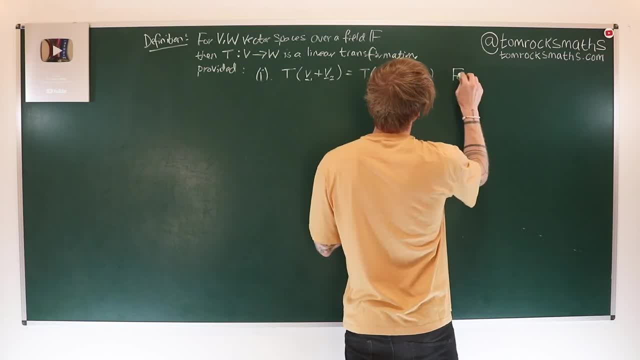 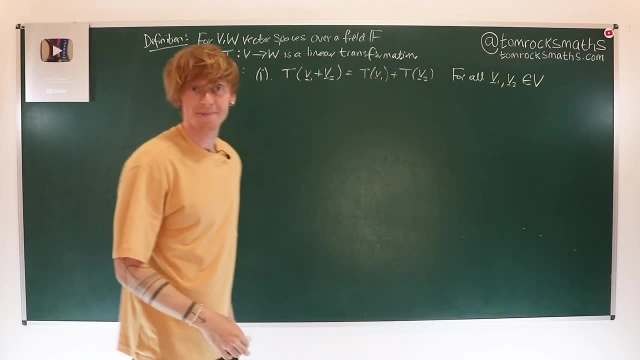 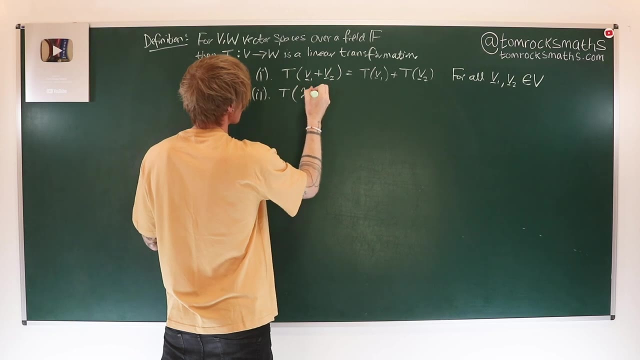 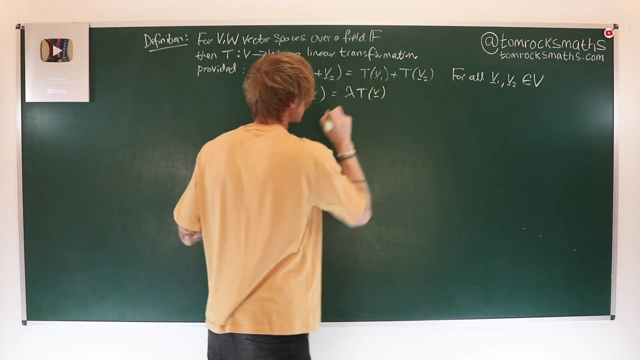 space V. So for all V1 and V2 belonging to our vector, space V. And the second property is that T of lambda times V must be equal to lambda of T of V, And this again needs to be true for all V and V2.. 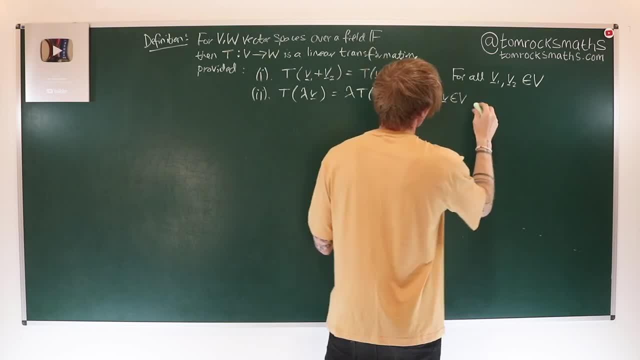 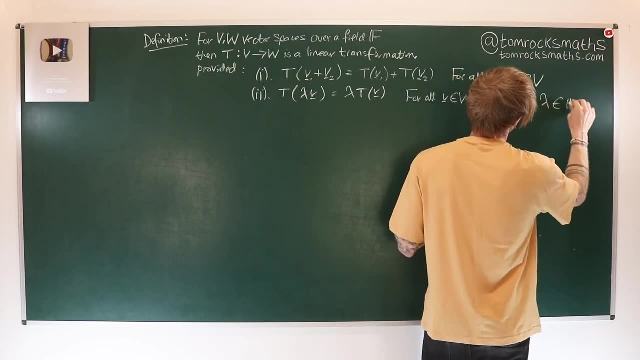 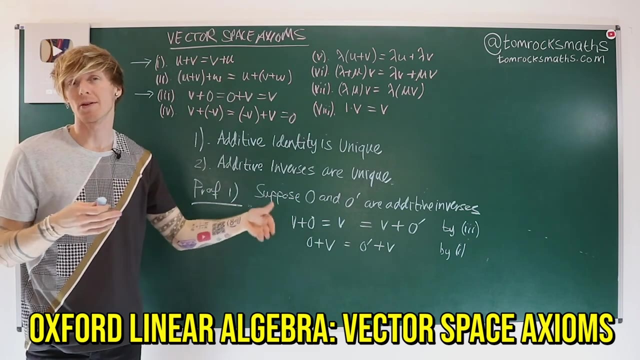 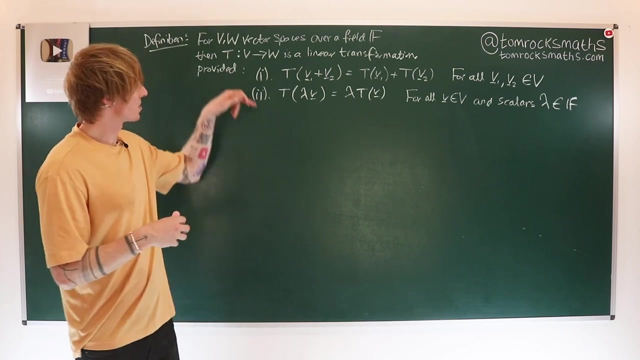 in our vector space: v, belonging to v, and scalar- scalar is lambda- belonging to our field. Now, if you think back to the full list of the vector space axioms, two things that were particularly important were the additivity property and what we're seeing here with 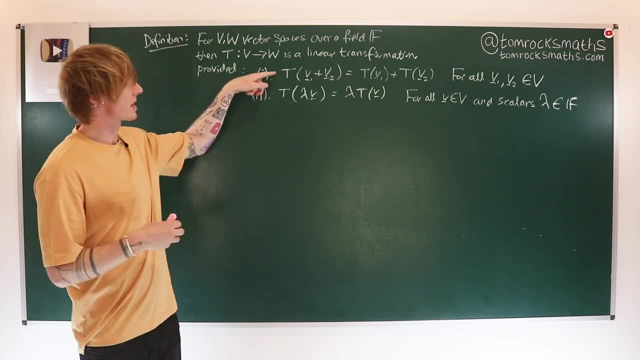 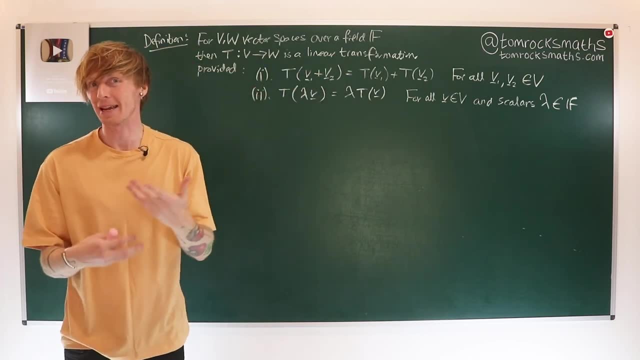 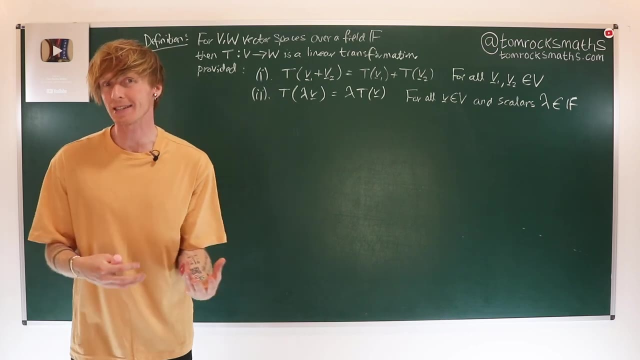 property one for a linear transformation is. this is ensuring the additive structure of the vector space is preserved when we do this linear map. And then property two is preserving the other important property we saw in the vector space axioms, and here that is scalar multiplication. 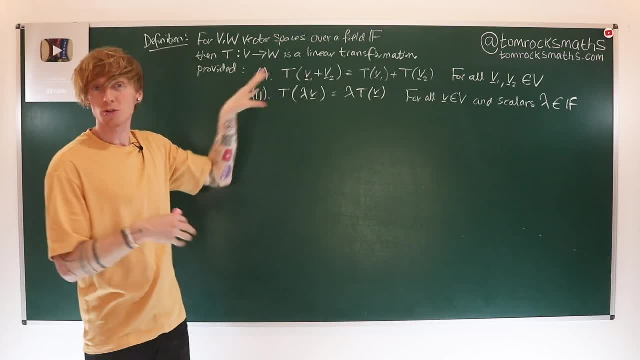 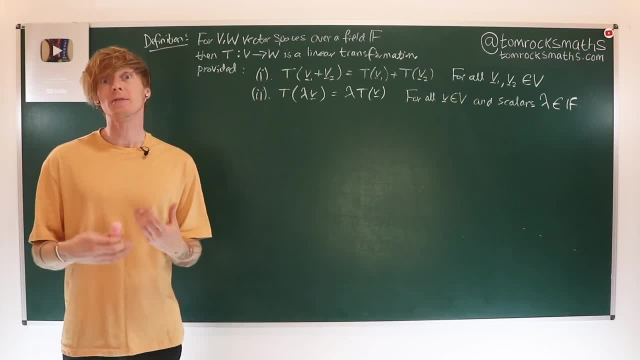 So, by ensuring that any map has these two properties, we are helping to ensure that map is preserved, To check whether a given map is indeed a linear transformation. we therefore have to check: does the map satisfy these two properties? Does it satisfy the definition? 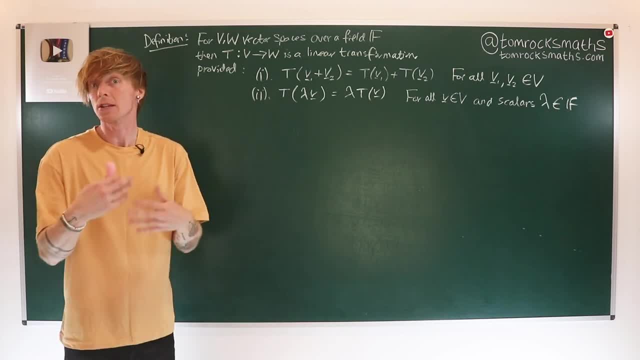 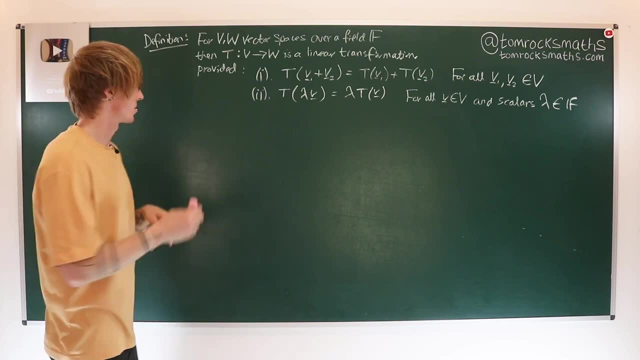 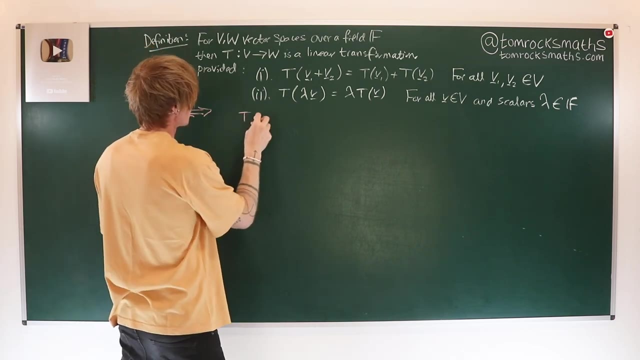 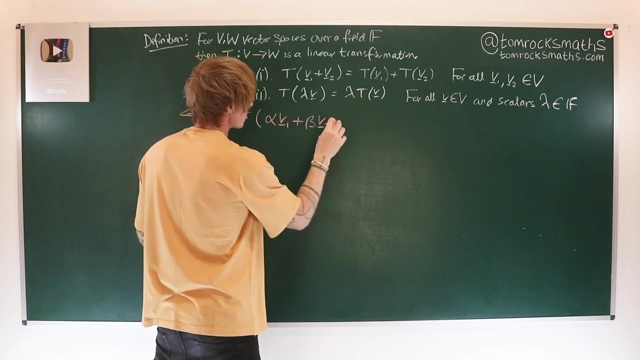 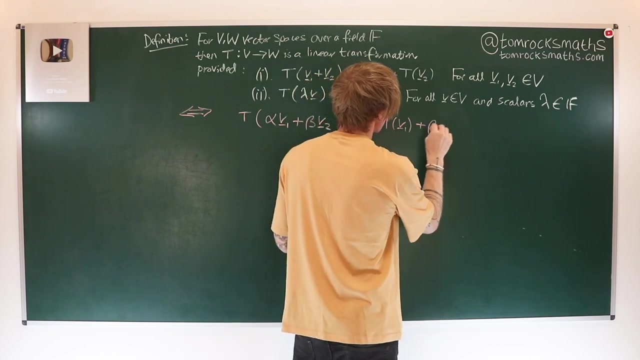 However, we can simplify things a little bit, in terms of checking potential maps at least, by actually combining these two properties. So this is actually equivalent to a single property holding, and that single property says that T of alpha times V1 plus beta times V2 has to be equal to alpha times T of V1 plus beta times T of V2.. 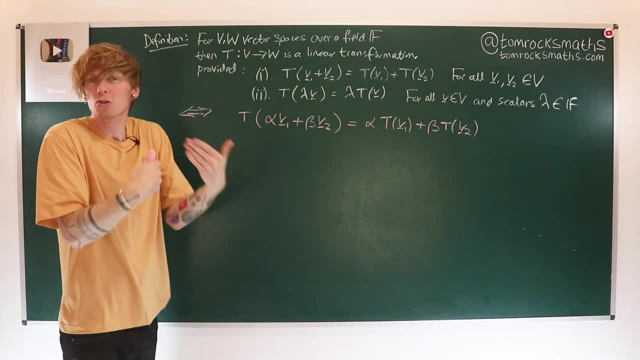 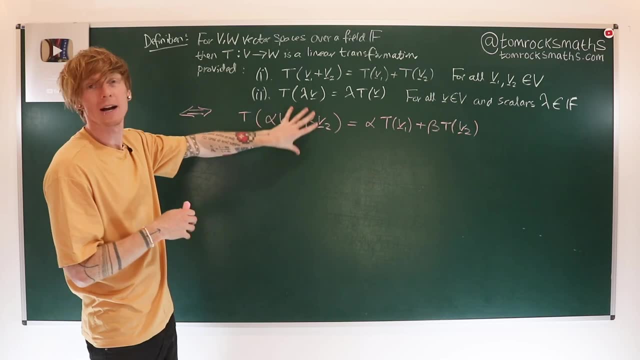 So if we can show this is true- and this is usually what is easier to check, because you're just combining, you're checking the two things at the same time, So it can save you a little bit of time to check this for a given map- and if this 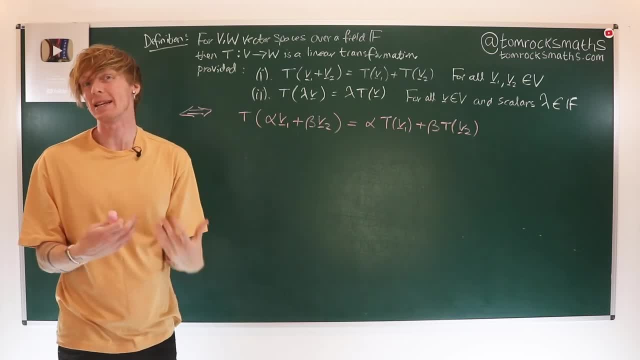 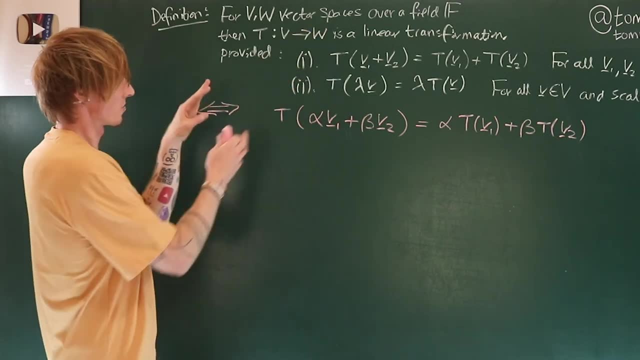 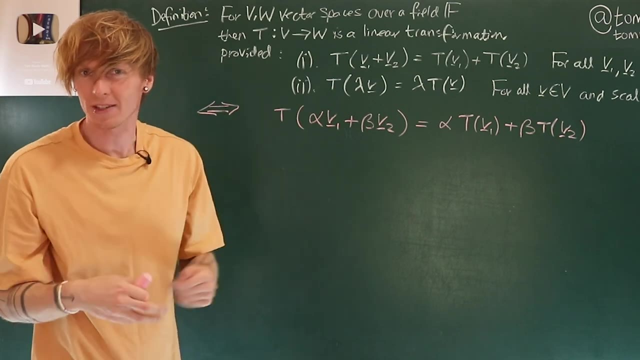 holds, then we can conclude that the map is indeed a linear transformation. Now to formally show that these are equivalent, we do need to check that. you can start either from the definition and get this condition, or start at this condition and get the definition. But it is relatively straightforward, so I'll just outline the 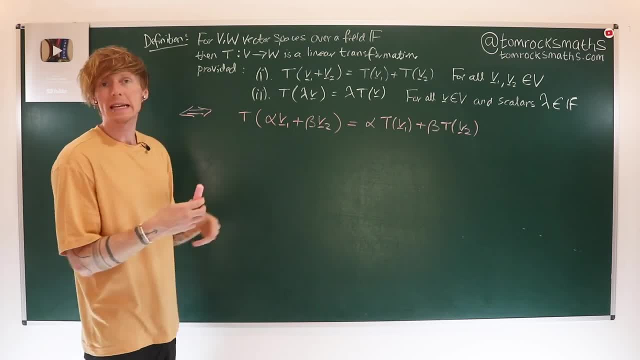 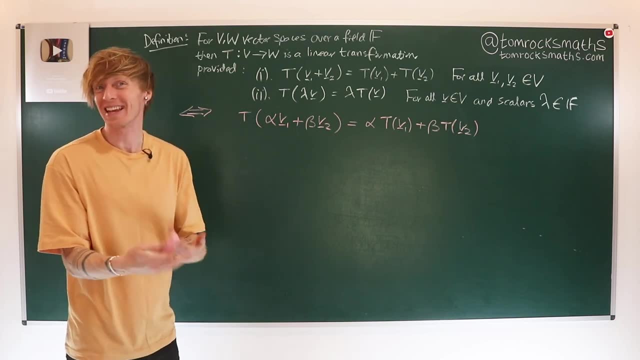 key steps. First thing to note here is: V1 is a vector in my space V. therefore any scalar multiple of V1 also belongs to the same vector space that follows from your vector space axiom. So therefore this is in V1, and so we can actually just 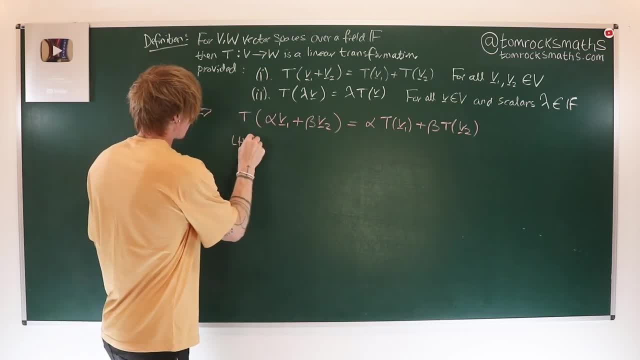 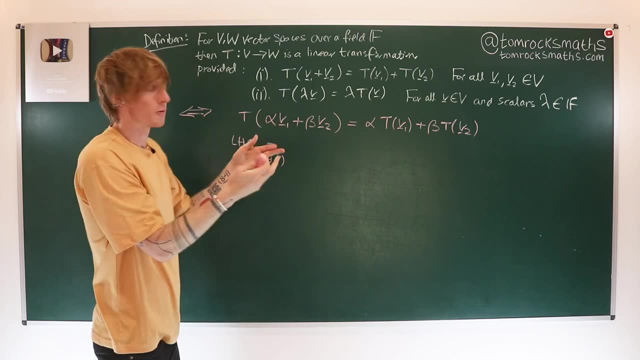 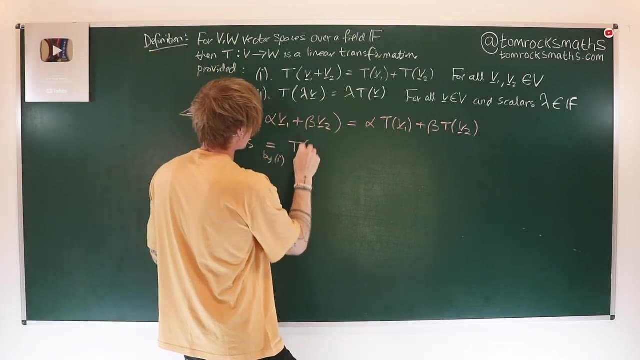 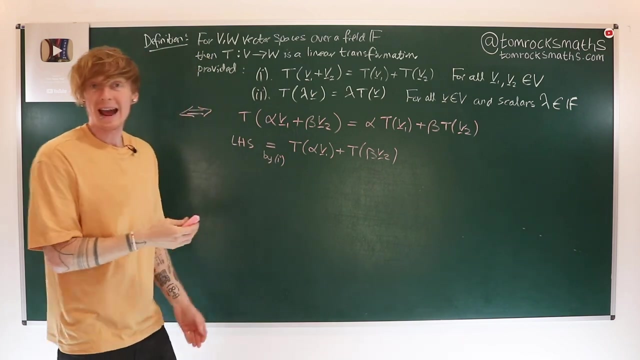 apply property 1.. So if we start from the left hand side and then by property 1, we can say: well, I can split this up into those two pieces, because each piece is a vector in the capital V, So alpha V1 plus T of beta V2, but now we have a scalar multiple inside and now we 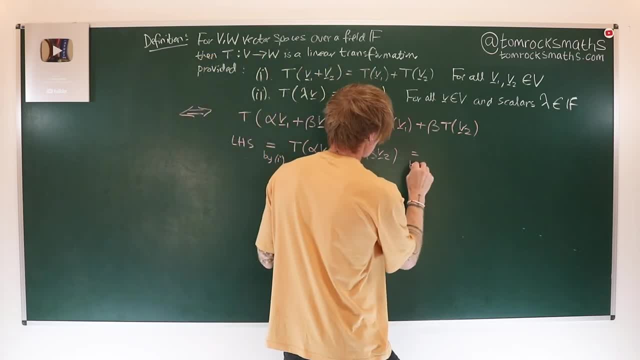 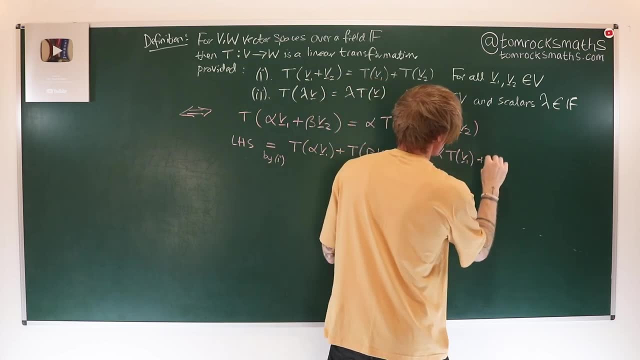 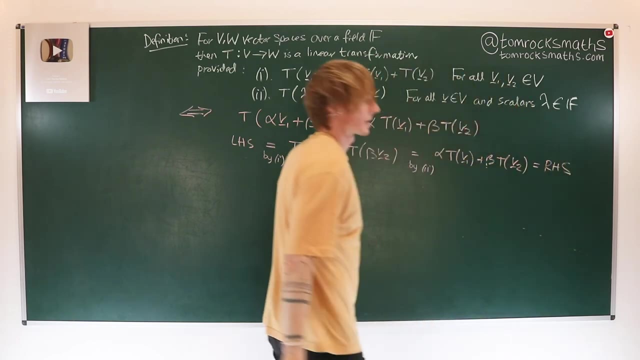 just apply property 2.. So now this is equal to by property 2, we can pull out the scalars, so it's alpha T of V1 plus beta T of V2, and this is of course equal to the right hand side. 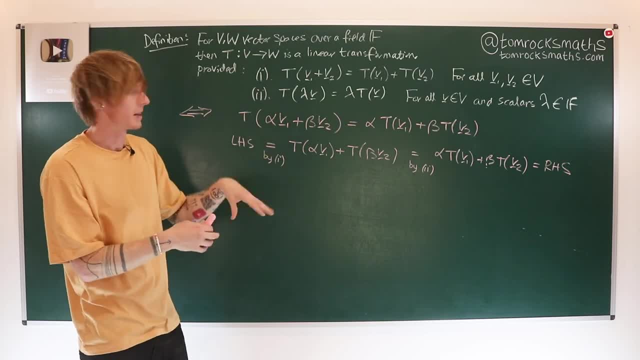 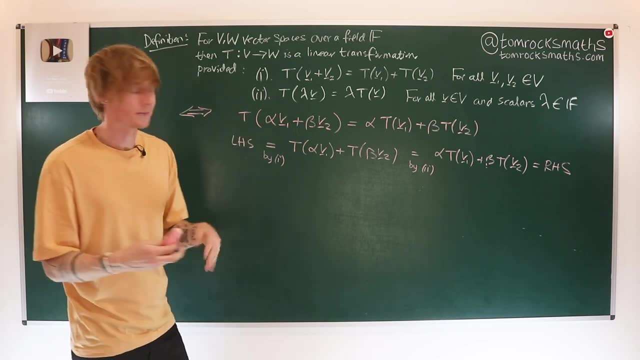 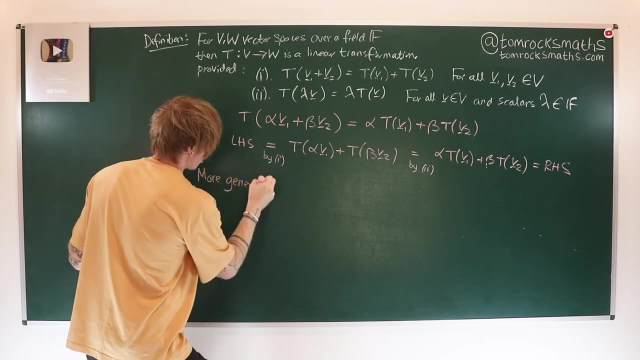 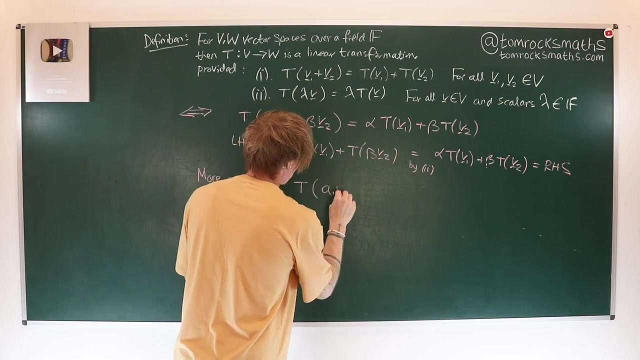 So we can see these two definitions are equivalent and that's why we usually use this one to test whether something is a linear map. And we can actually go even further and sort of more generally, we can say: in fact, y, stop at 2.. If we have a linear map, then in fact T of a1, V1 plus a2, V2 plus. 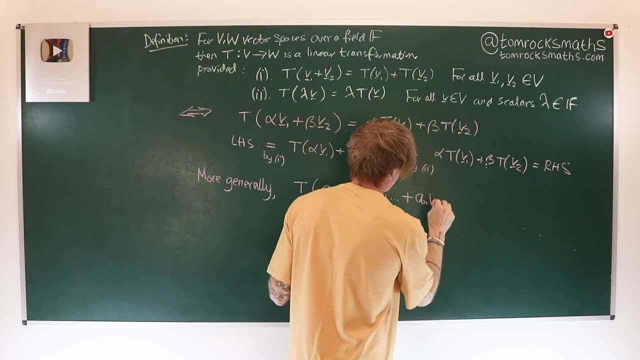 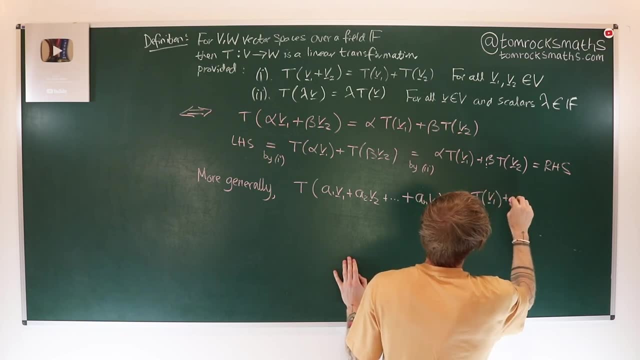 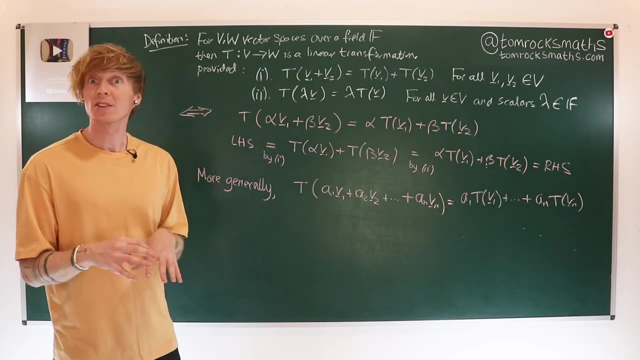 all the way up to an vn is indeed going to be equal to a1 T of v1 plus dot, dot, dot plus a n T of vn, And this version is going to be particularly helpful, as we will see in the next video. 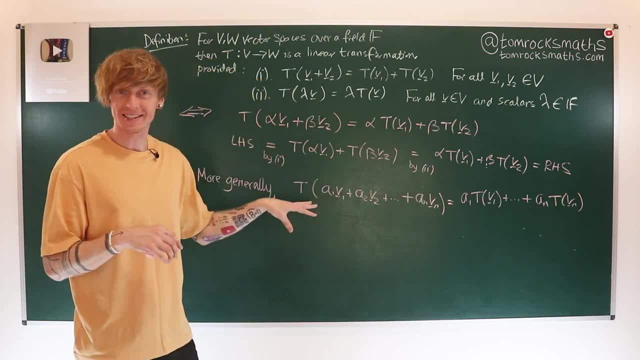 when we start talking about bases of vector spaces, because, as we've seen in previous videos, if v1 to vn were equal to a1 T of v1 plus dot, dot, dot plus a n T of vn, then this version is going to be particularly helpful, as we will see in the next video when we start. 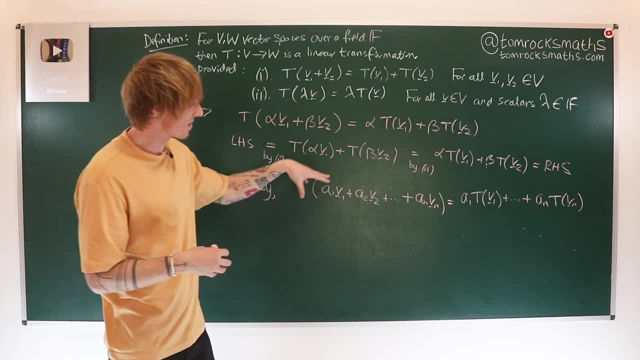 talking about bases of vector spaces because, as we'll see in the next video, when we start talking about bases of vector spaces, if vn were to be a basis of my vector space, then any vector in that space must be able to be expressed as such a linear combination of. 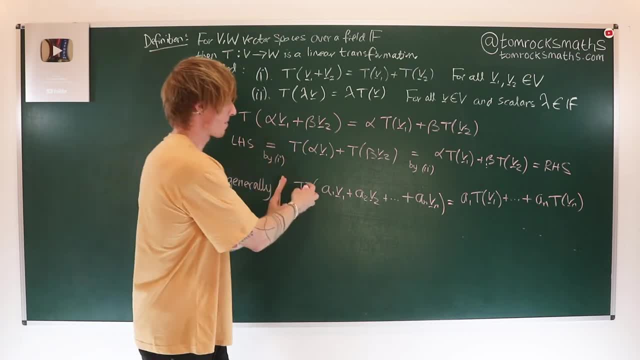 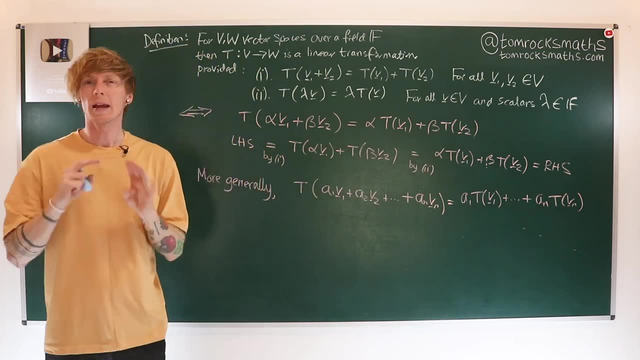 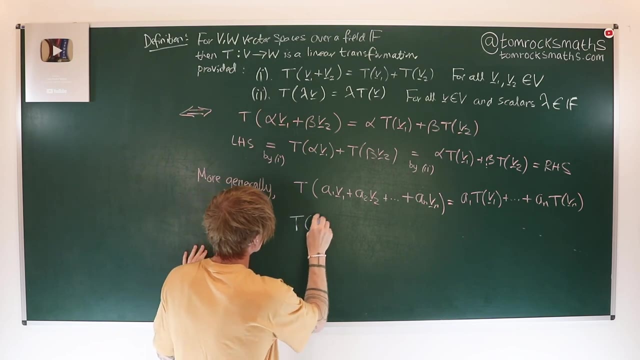 the bases vectors, and this is telling us how a linear map would act on, therefore, any vector from that space. But more on that in the next video. Another important property of a linear transformation is the following: T of the 0 vector has to: 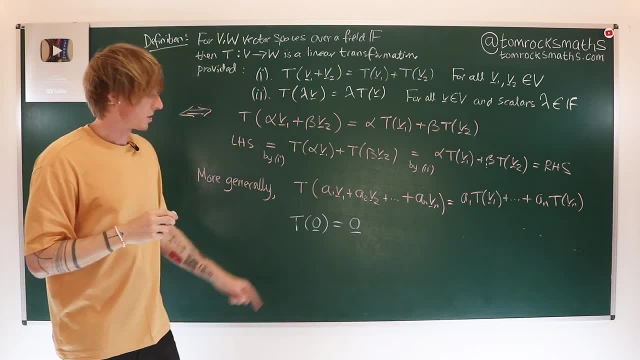 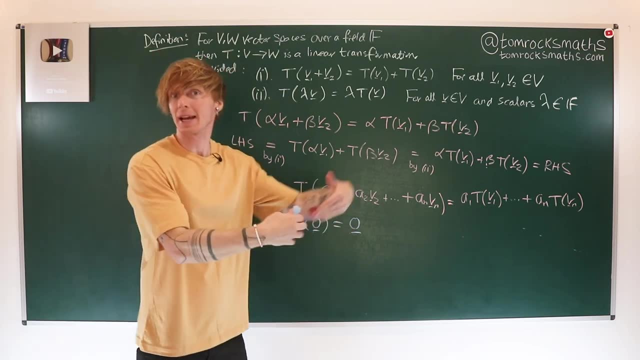 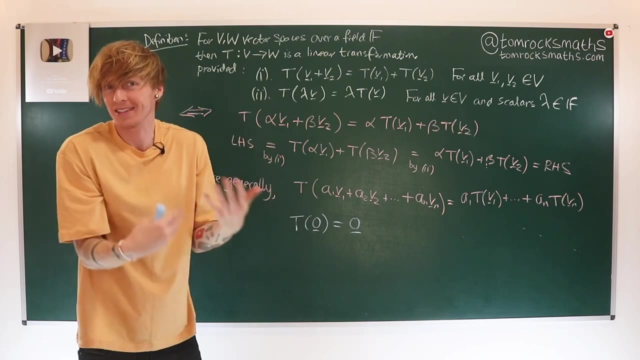 be equal to 0.. to the zero vector. So this is the zero vector belonging to my starting space V, and this is the zero vector in the space I end up in, the space W up here. So both vector spaces have to have a zero, because that is one of the axioms of 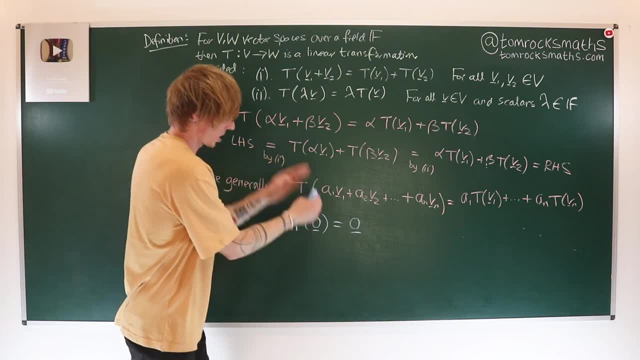 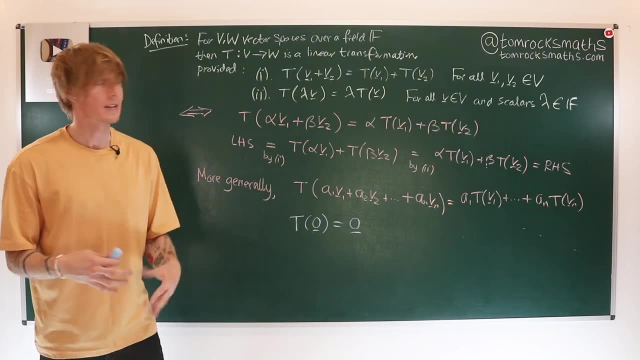 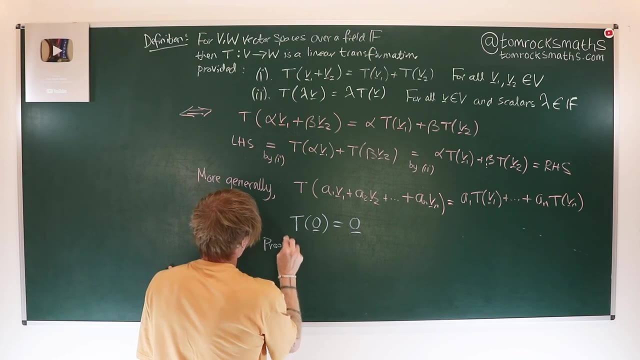 being a vector space and this is saying if we start at zero and apply t, we have to get zero in the new space. The proof here is quite straightforward. it just pretty much follows from property one in our definition, but I will sketch it out regardless Proof. So if we consider 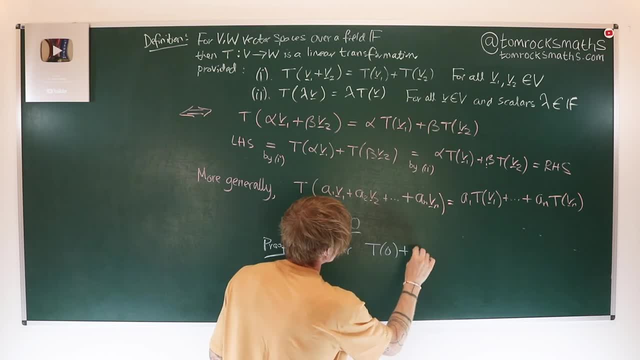 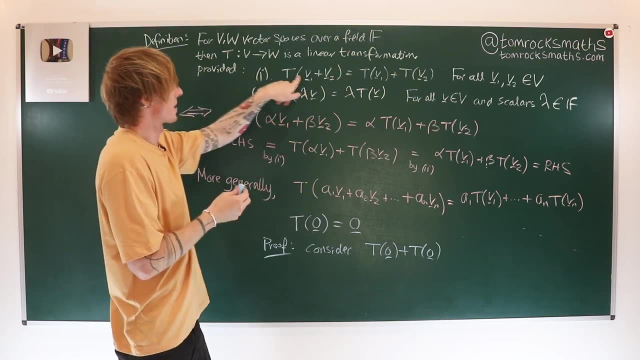 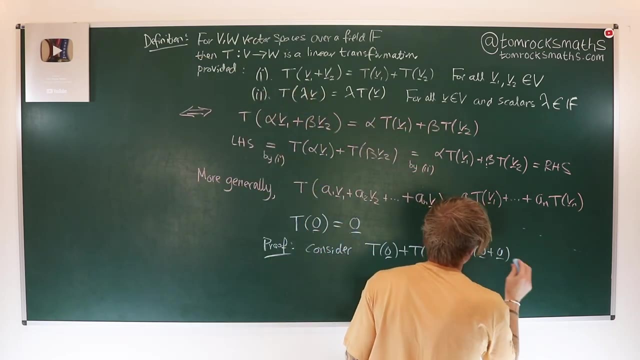 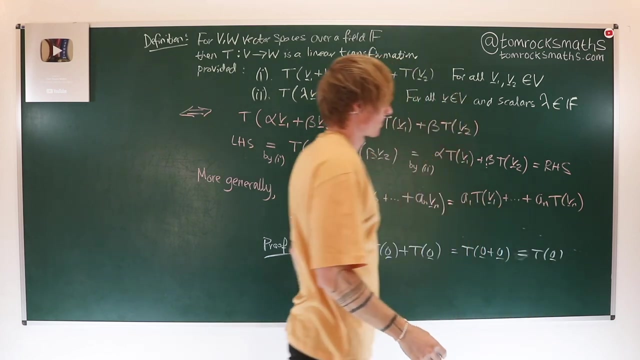 T of zero plus T of zero. then by property one, this is the same as T of zero plus zero. so this equals T of zero plus zero. but of course when you add zero to something you just get back zero, so that's just T. So now we've got two lots of T equal to T. so 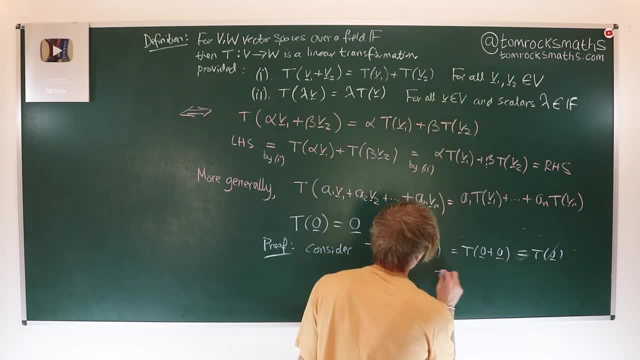 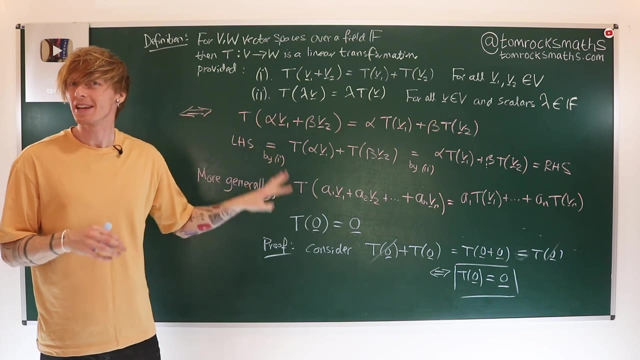 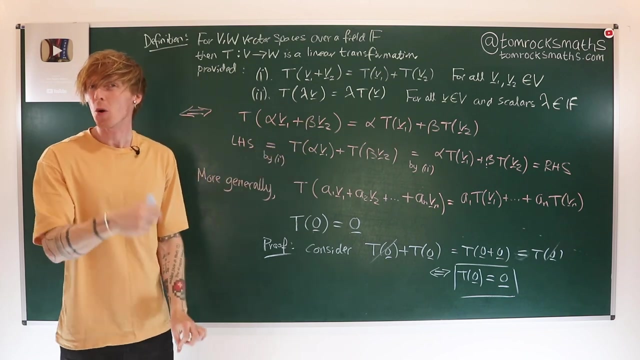 we just cancel that on each side, and that's basically therefore saying that T is equal to naught. This is, in fact, a very useful property, so I would recommend noting this one down and committing this to memory, as showing that this doesn't hold is a very quick way to show that a given map is not a. 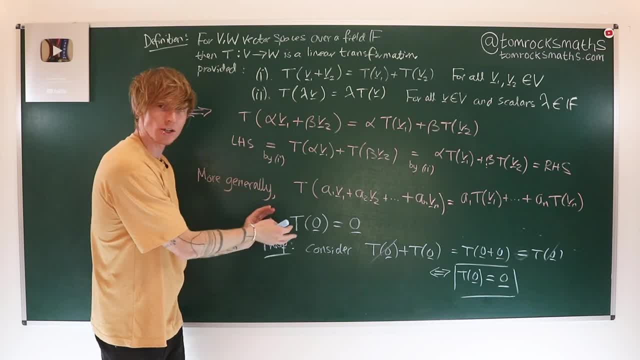 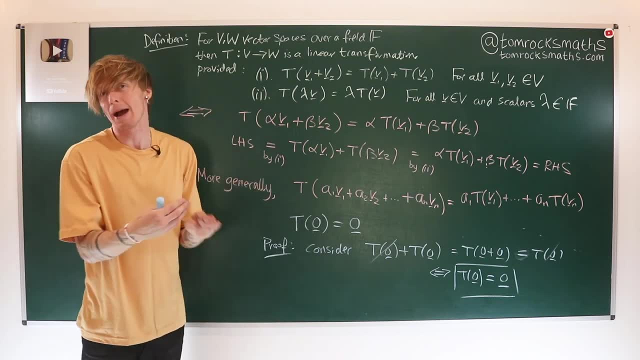 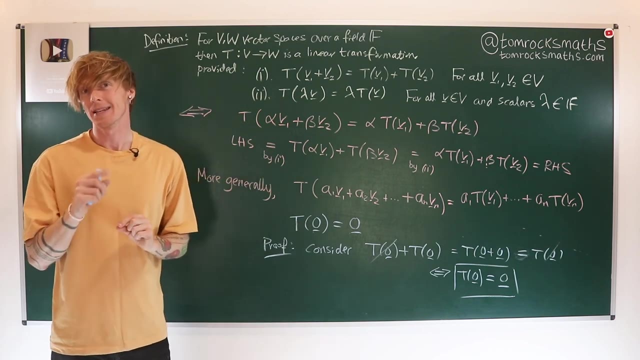 linear transformation. So if this does hold, it doesn't mean your map has to be a linear transformation. There are examples where this is true, but the map will not be linear. However, if this does not hold, your map cannot be linear, be a linear transformation, and I will actually use this on some of our 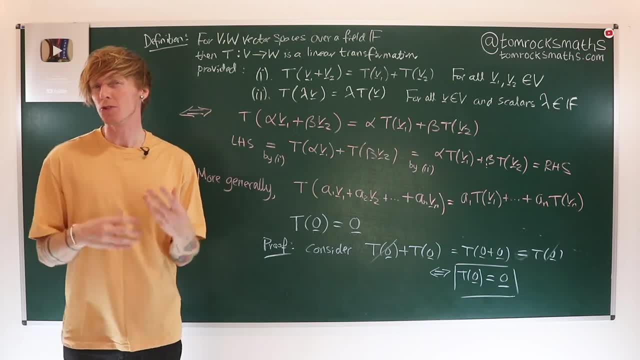 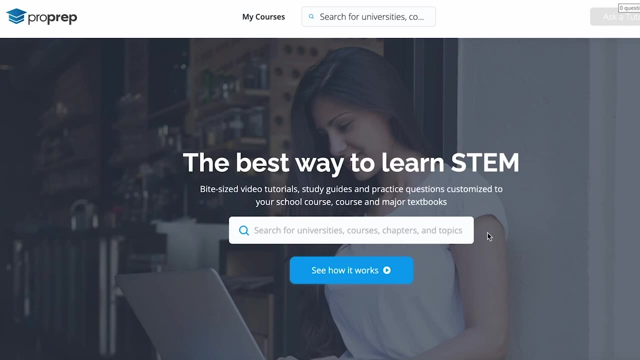 examples which will be coming up shortly. Now, before we do move on to look at those examples, now is actually the perfect time for you to head over to ProPrep for additional explanation videos looking at the topic of linear transformations. ProPrep is an online resource which uses video tutorials to 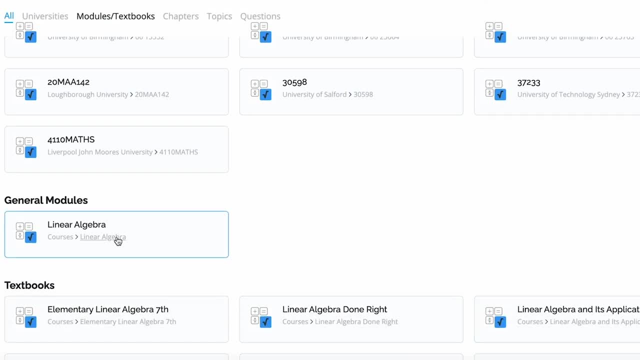 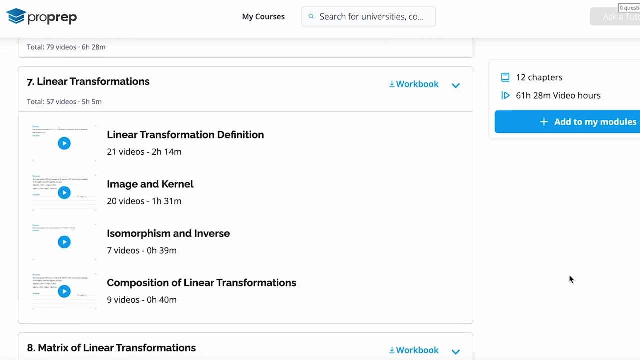 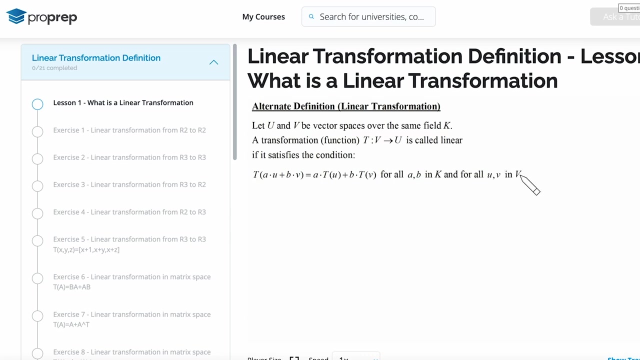 help students to improve their skills in stem-based subjects. Within the linear algebra module, you can find an entire section devoted to linear transformations. The first video provides a short lesson introducing the definition, just as I've done in the video so far, before moving on to some 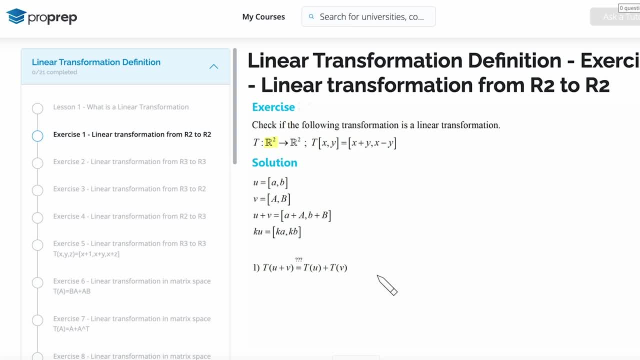 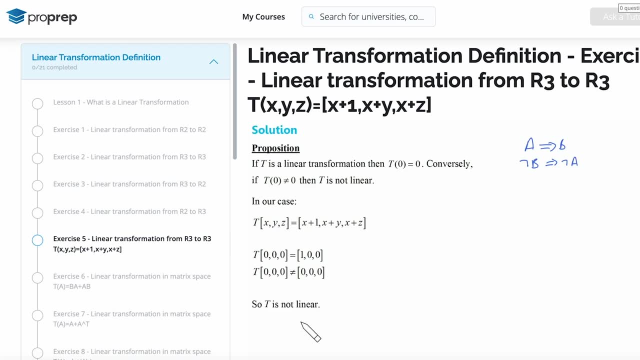 fully worked examples and then a further 20 videos covering a whole range of exercises, each one with its own complete video solution. You'll find examples for n-dimensional vectors, n by n, real matrices and linear transformations, If you're interested in learning more about linear. 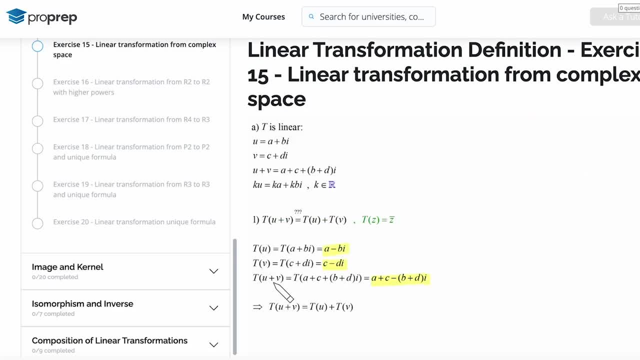 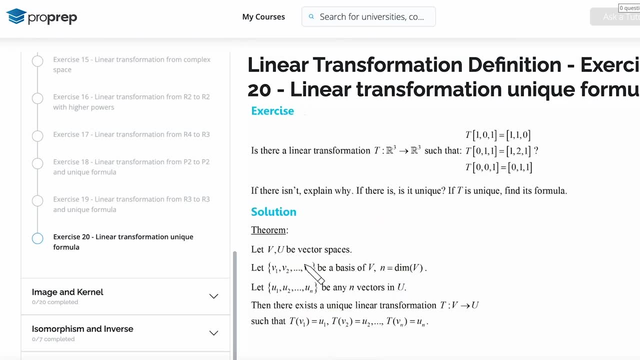 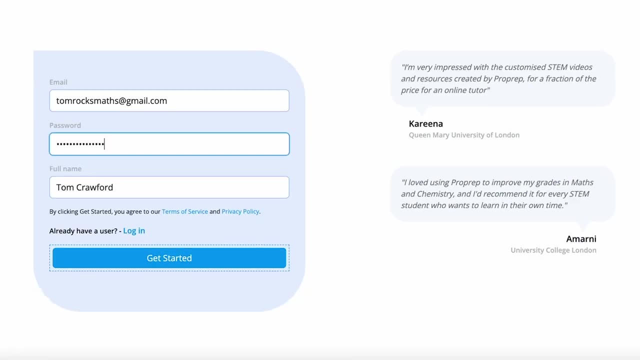 transformations. you can click on the link in the video description For full access to all of the videos. you can sign up for a 30-day free trial, courtesy of Tom Rocks Maths, by clicking on the link in the video description. Get started now and take your learning to the next level. For our first example, we're going to 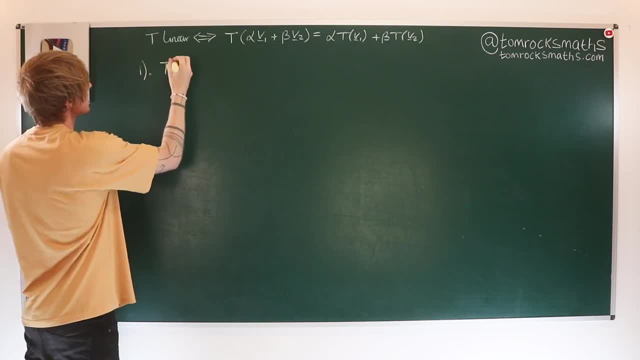 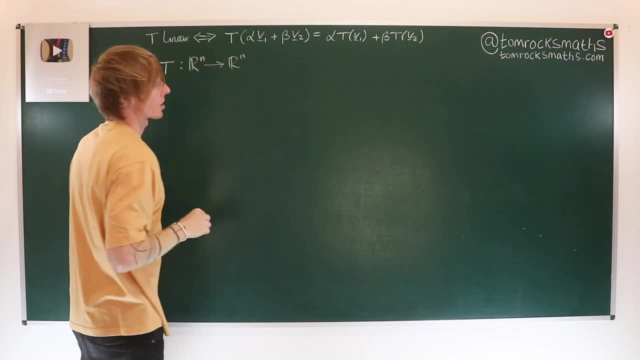 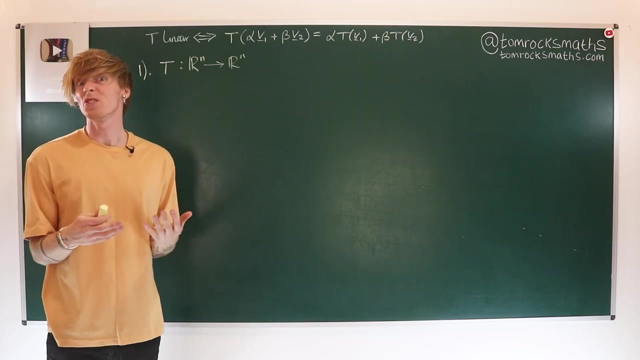 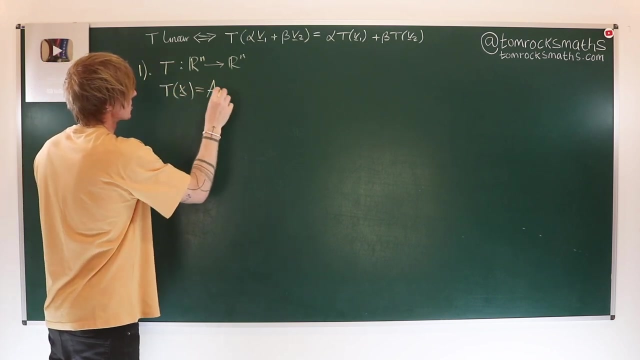 look at a map T which goes from Rn to Rn. It's going to do so via multiplication by an n, by n matrix. let's call it a. So if we were to input a vector X, then T of X would give us a, which is our matrix times. 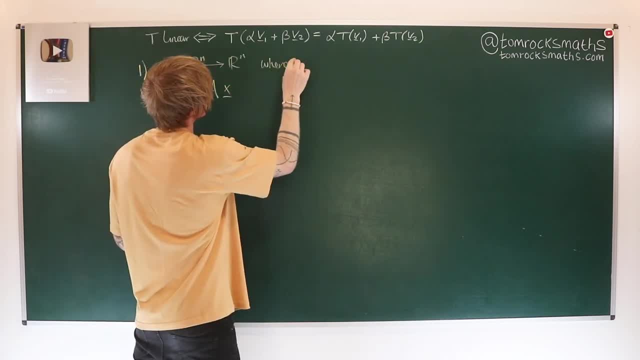 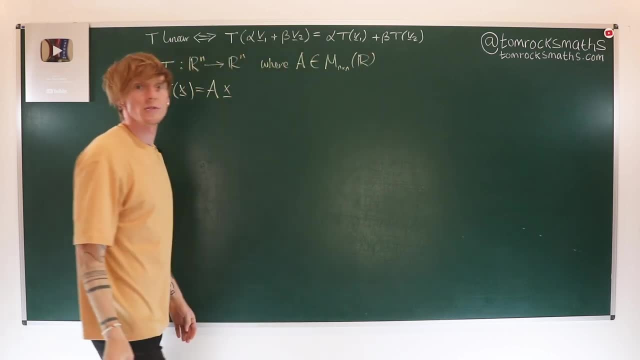 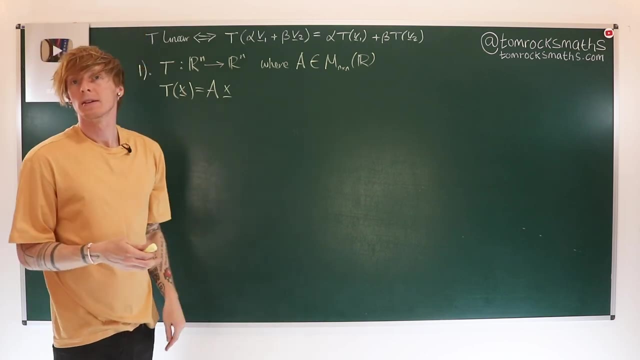 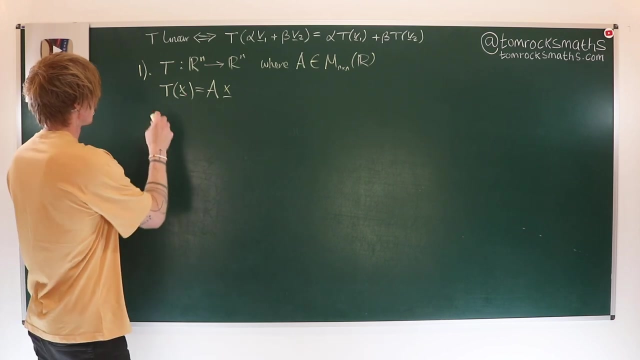 X, and I'll just say where a belongs to, the n by n matrices with real entries. So we want to check: does this define a linear map? I've written our definition, as it were, at the top of the board, so we just need to check if this is going to be true. So we 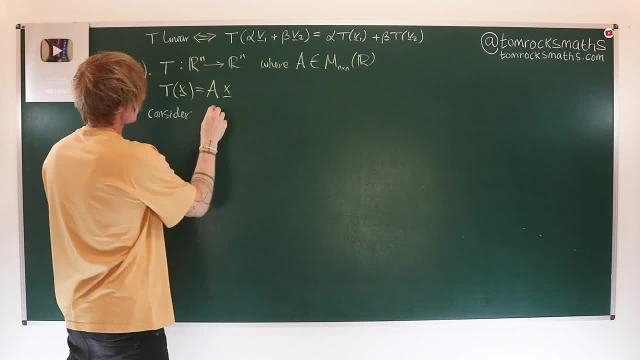 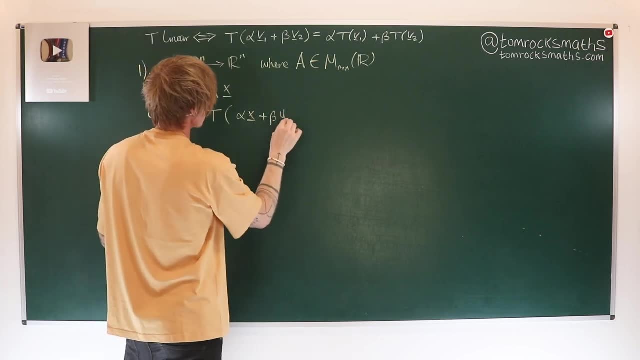 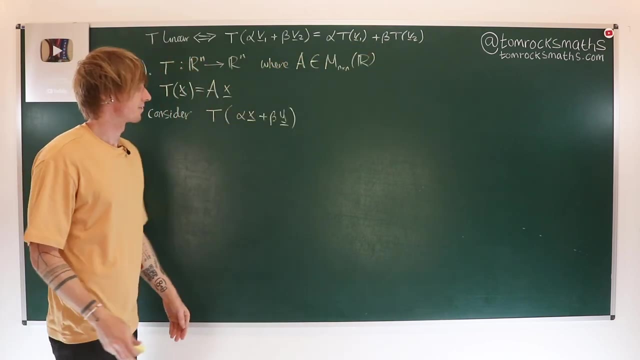 need to consider, therefore, T of a constant. let's go with alpha times x plus beta times y, and we need to show that's the same as these two individual pieces added together. So if we apply our map, we just get a left multiplying the whole. 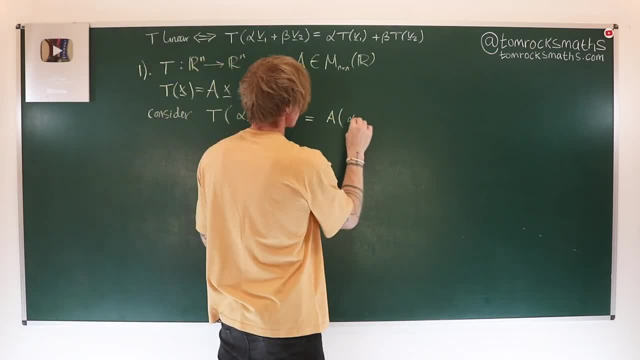 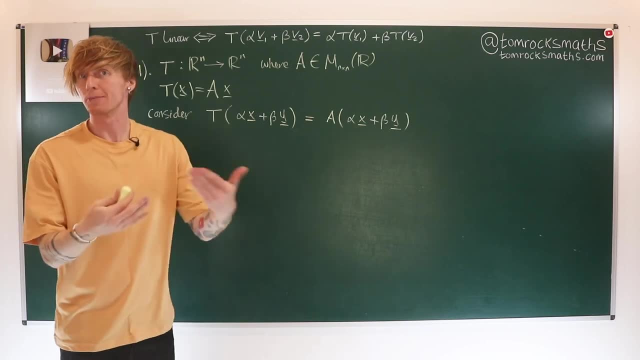 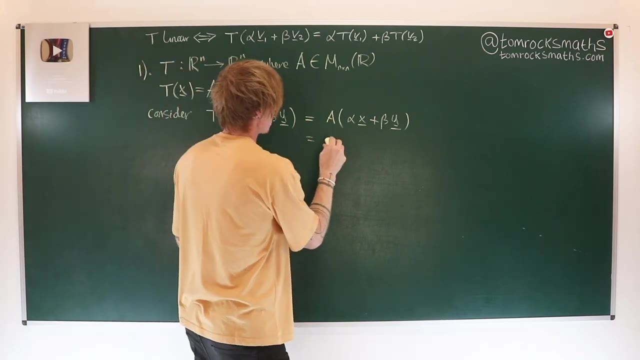 thing. so that's just then a times the input, which is alpha x plus beta y, and now we just use the properties of matrix multiplication. So we know that if we have a scalar we can pull that out in front of the matrix. so that's going to. 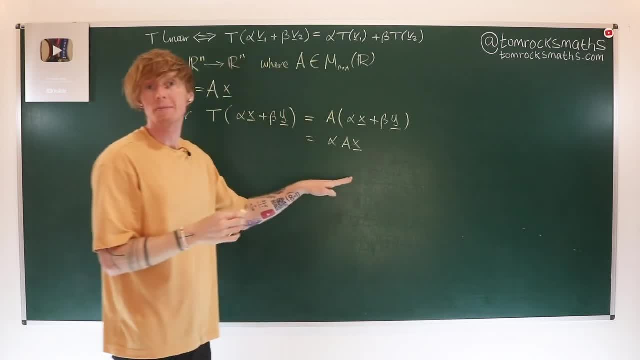 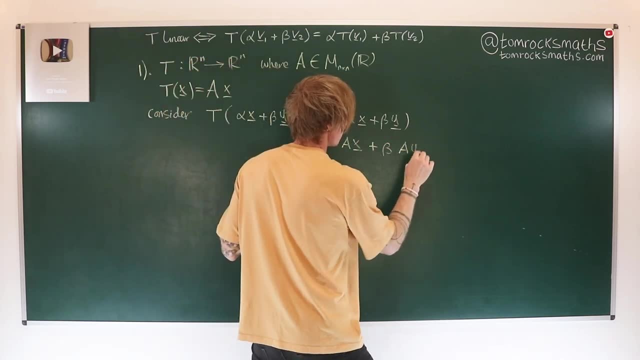 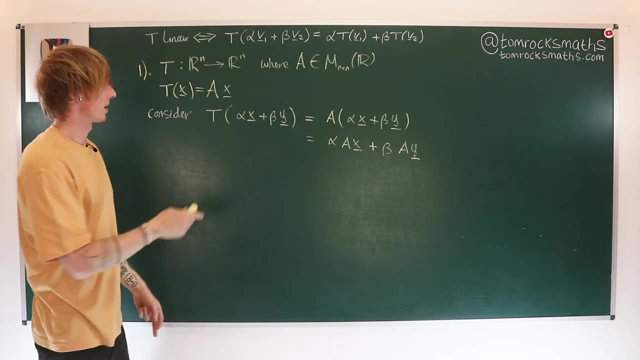 be alpha, then it has to be a x. we have to keep them in the correct order, of course, and then we can pull out the beta, and then we've got a y. But now, if we think about, what are these individual pieces? well, if I were to 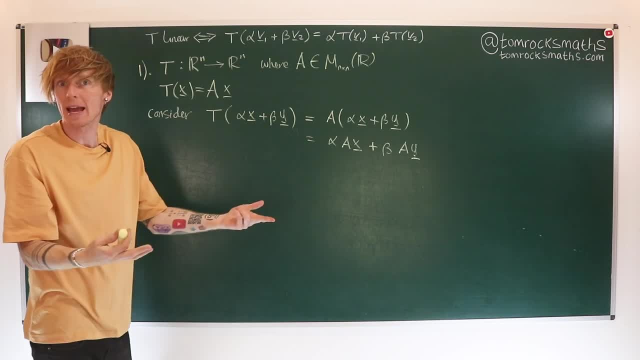 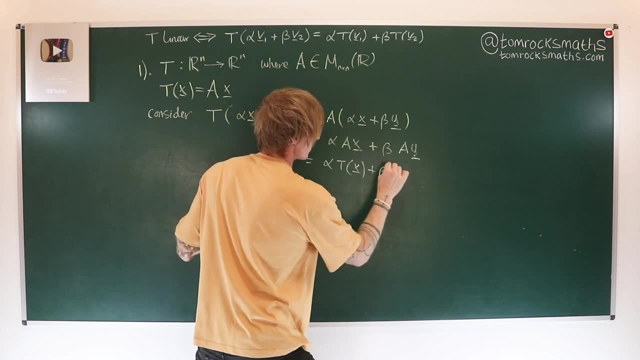 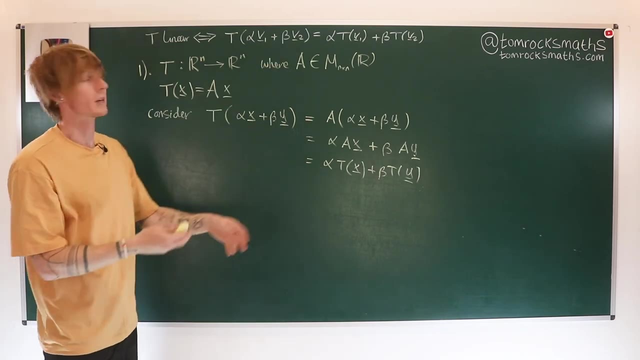 apply T to x, that gives me a x. So this is actually just alpha times T of x plus beta times T of y, and this is exactly what we needed to show at the top of the board. So we can conclude this map. multiplying a vector by a matrix is indeed a linear. 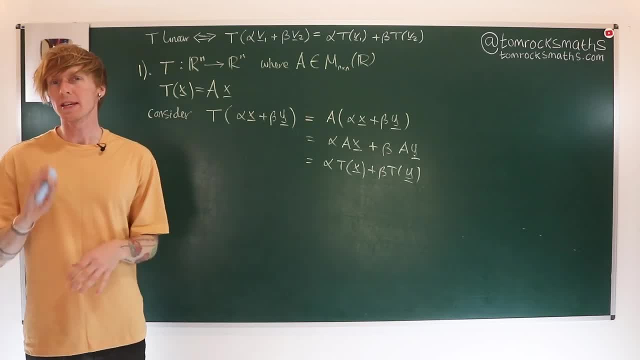 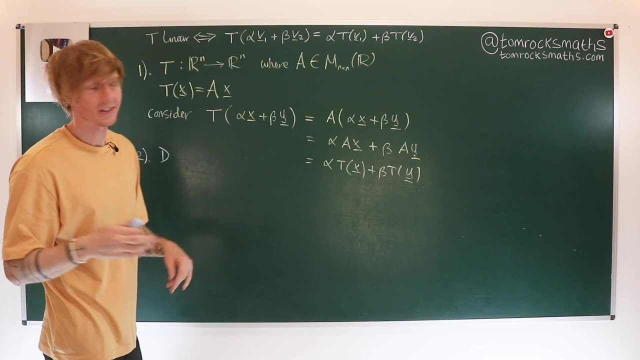 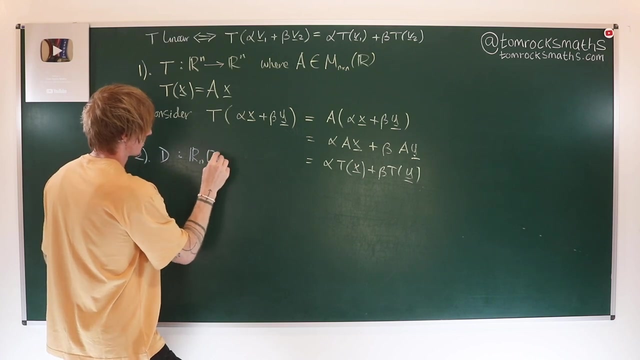 transformation. Let's look at another example. This time we're going to suppose we have a map D and D is going to be differentiation, So D is going to map from the. let's suppose they are real valued polynomials up to degree n. So we: 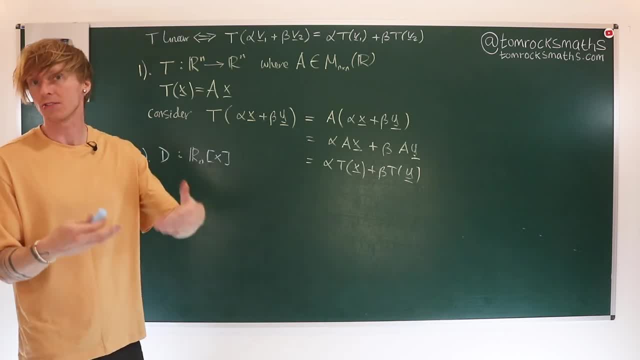 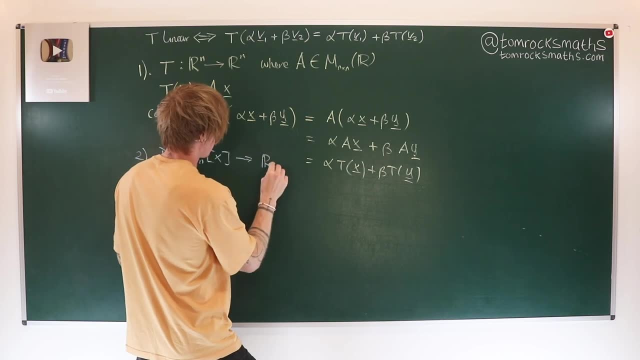 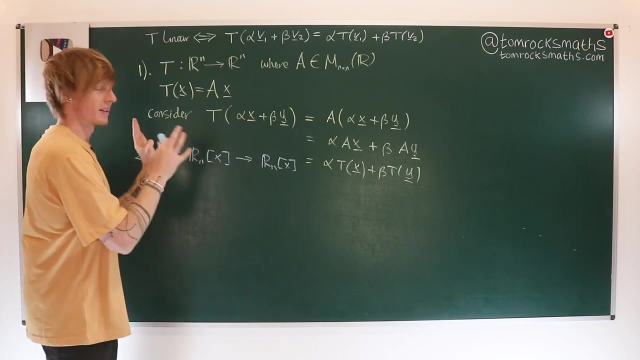 have seen this space before in some of our earlier videos in the Oxford linear algebra series. So Rn, and it's going to output into the same vector space. Technically the output would be for, but that's ok because that is going to be a subspace of the one I've 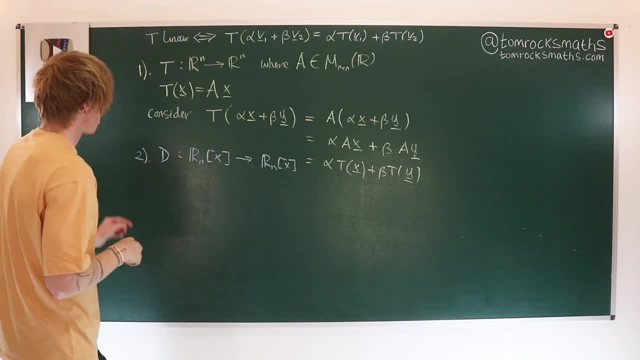 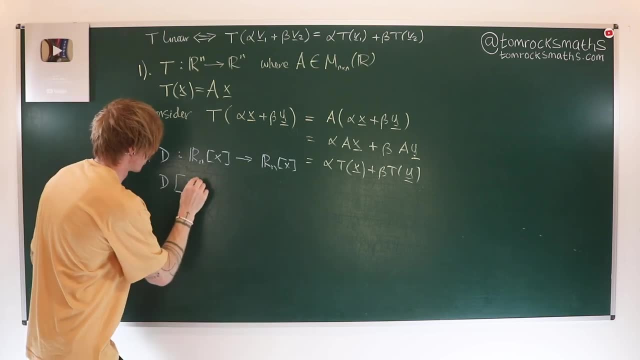 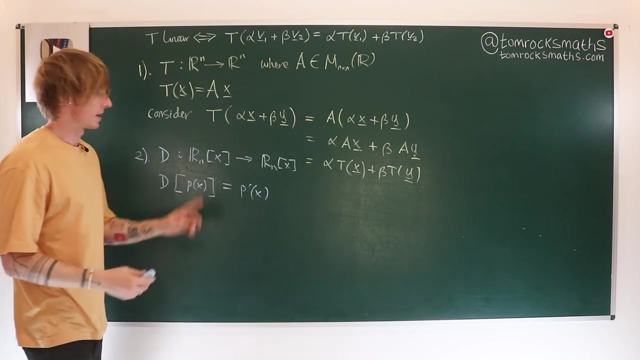 written here. so this is still true. The map is going to work by saying that D of a polynomial. So let's suppose we input P is going to output its derivative p prime of x, and this is where p is of course a polynomial in x, with a maximum degree up to n. So if we take the most, 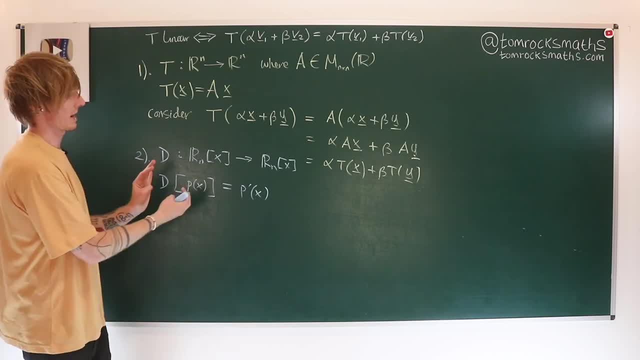 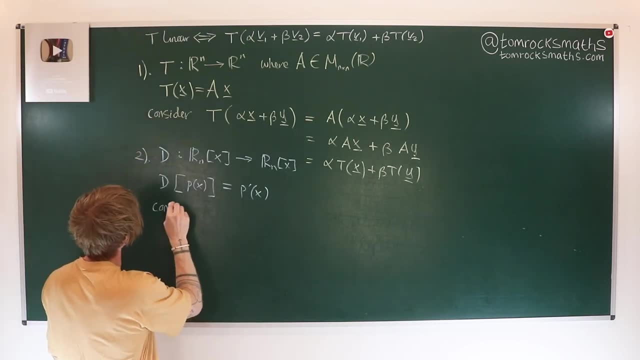 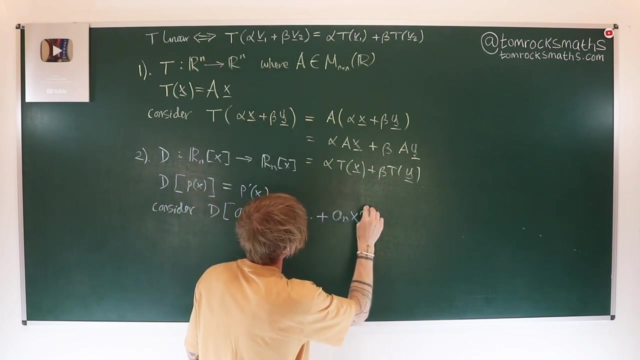 general form of p. we need to show that this is indeed linear, as defined at the top of the board. So we're going to consider, as I say, the most general polynomial, which is going to be a0 plus a1x plus dot, dot, dot up to an times x to the power n. Now the map d is differentiation. so if 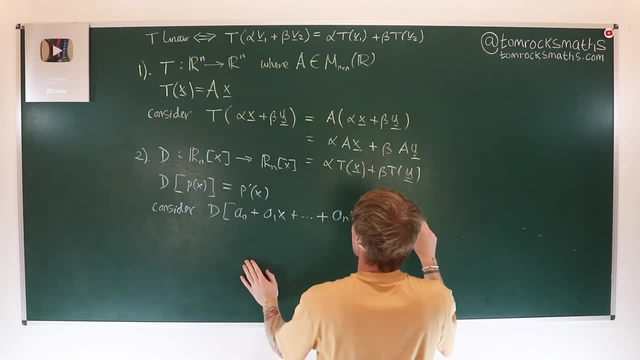 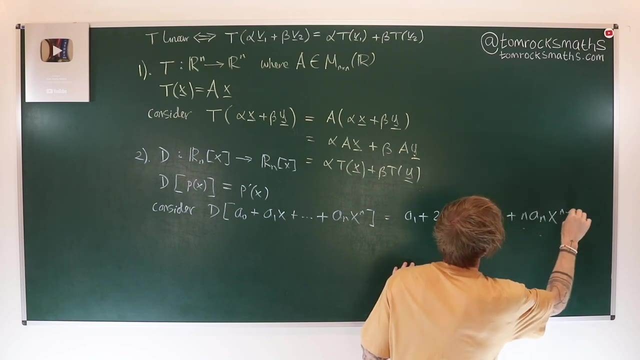 we apply that, then we're going to get a1 plus. we would then have 2a2 times X and then all of these sort of bits and the middle, and then the last piece is going to be n times x. I think the. 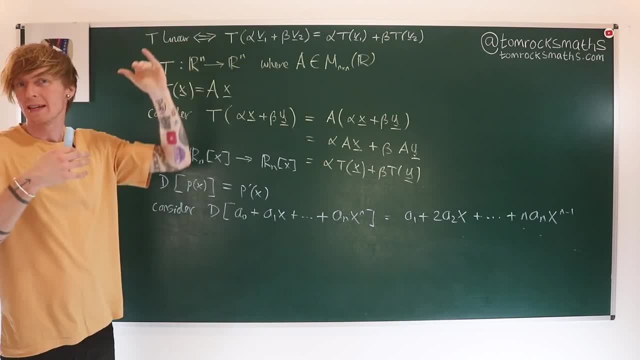 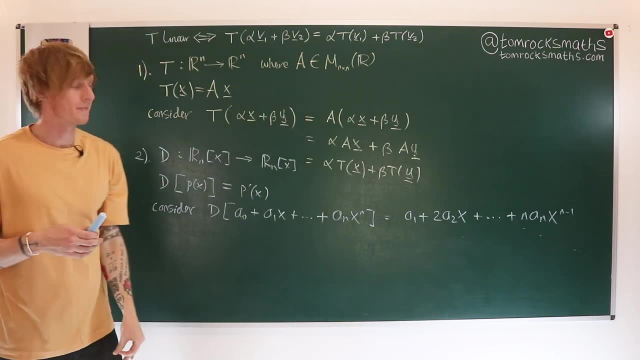 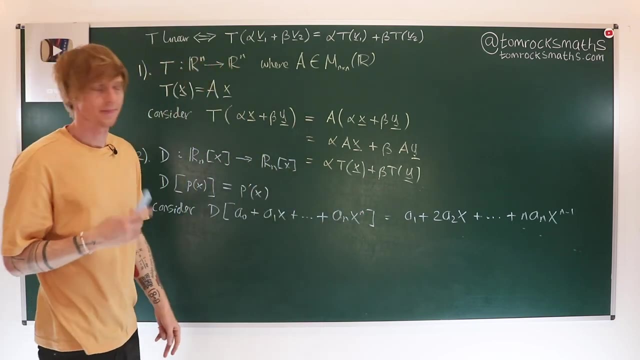 easiest way to show the linear transformation definition is satisfied is actually to now consider the right-hand side of our expression up here in the notation of this question and show that we get the same thing that we have here. So we've done it one way. this is like the left-hand side of our 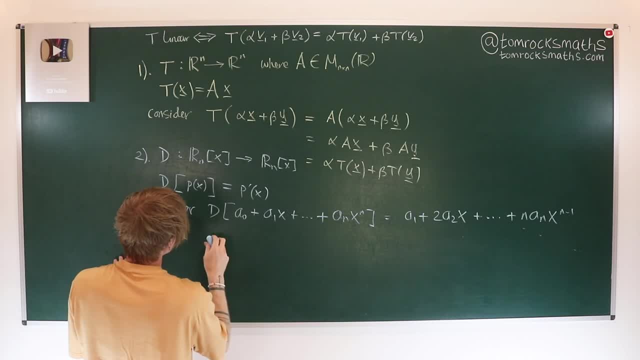 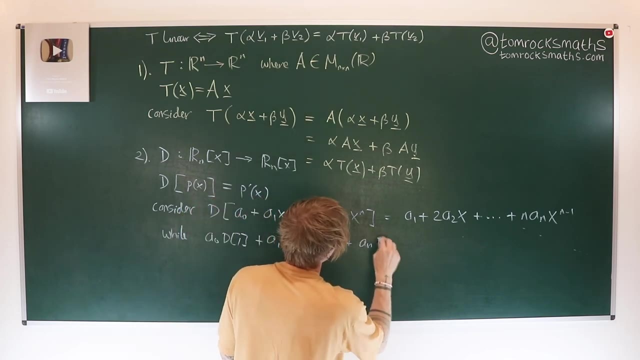 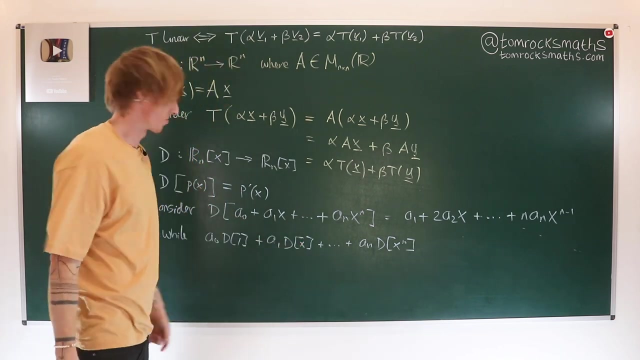 definition. so if I now consider it piece by piece, then I need to pull out the constants. so I need a nought times d of one plus a, one times d of x, plus dot, dot, dot, up to a n times d of x, n. But given we know how differentiation works, this is: 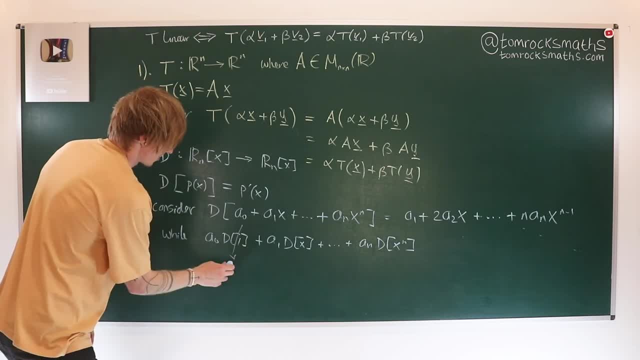 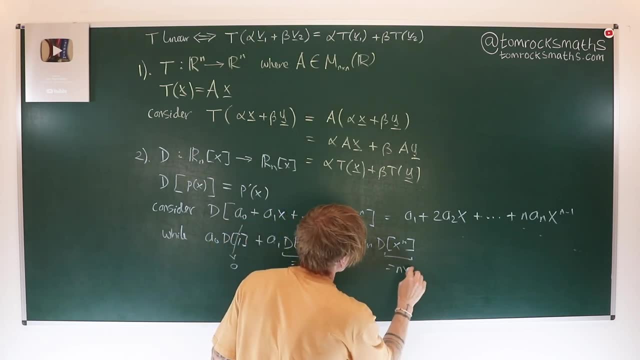 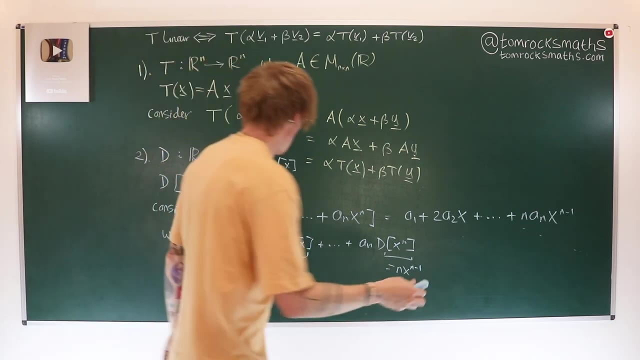 of course going to work in the same way. So this gives me zero. the derivative of x here, this is just one. the derivative of x to the n is n times x, n minus one. so actually applying the map, now d, the differentiation map, I can say well that. 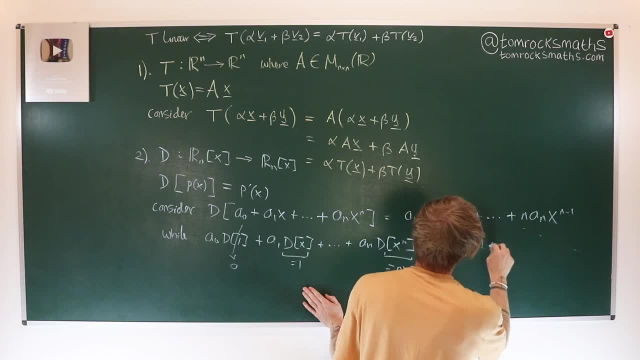 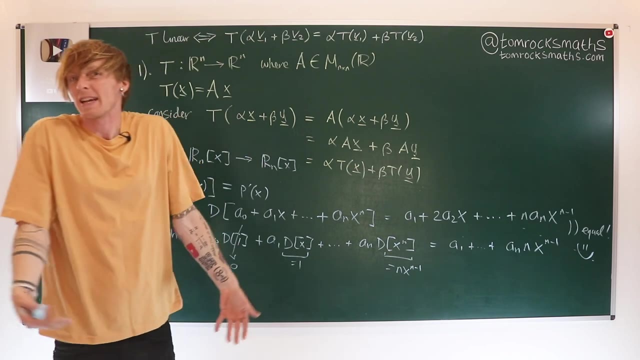 one disappears and then I'm left with a one plus all the bits in the middle, and at the end I've got a n times n, x, n minus one, which of course they are equal. Smiley face. So we probably expected the differentiation map to be linear. 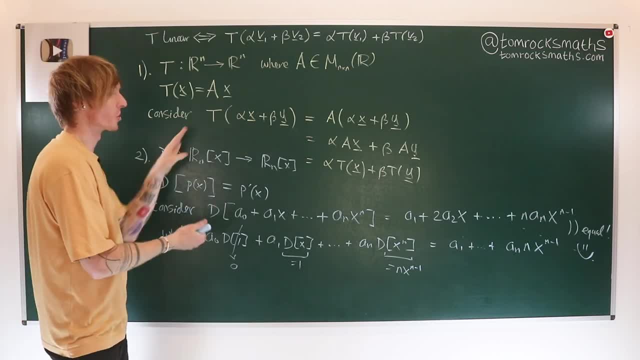 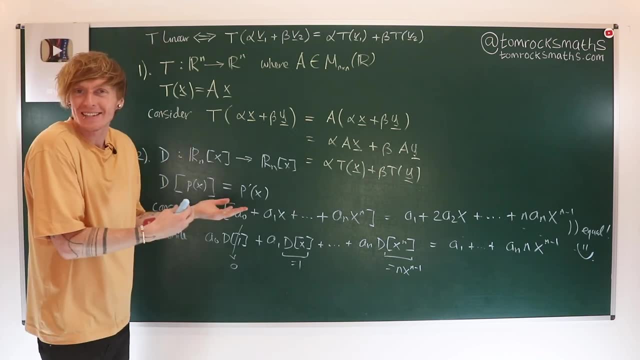 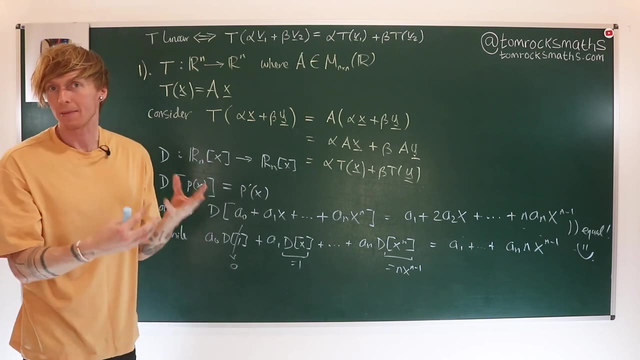 because when you study it in calculus, we show that it is indeed a linear operator in the setting of calculus. So it would make sense- and, as we see, it is true that it is also a linear map in this new setting, talking about linear. 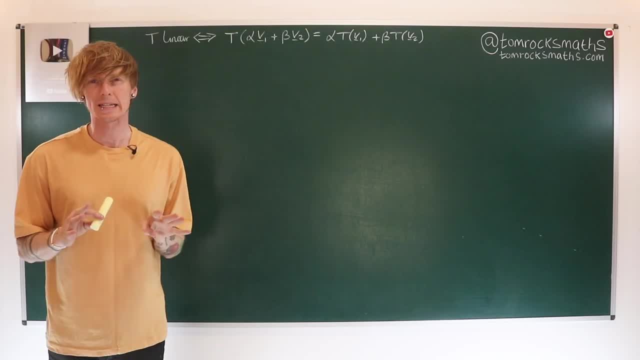 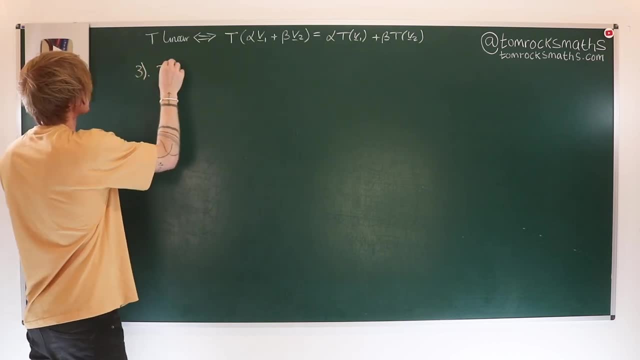 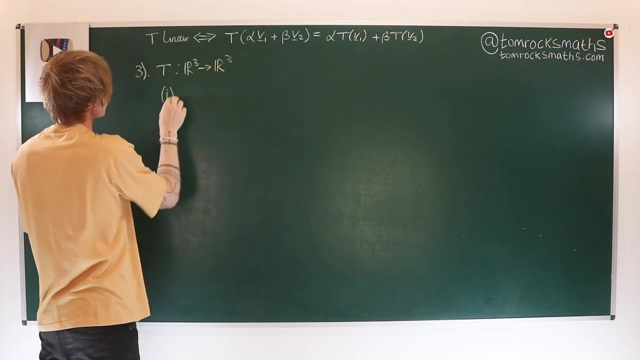 transformations, vector spaces and linear algebra. For our next example, let's make things a little more explicit. So we're going to be working with a series of maps t which are going to go from r3 to r3.. Let's suppose the first one, if you. 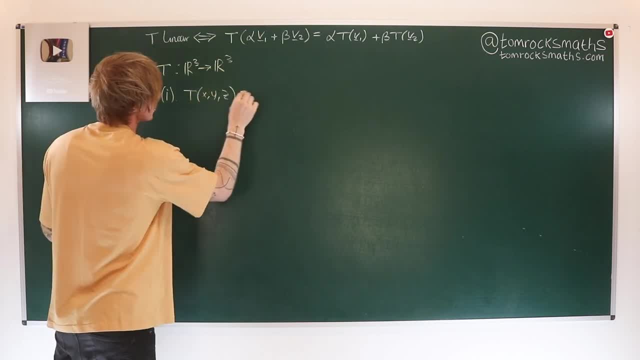 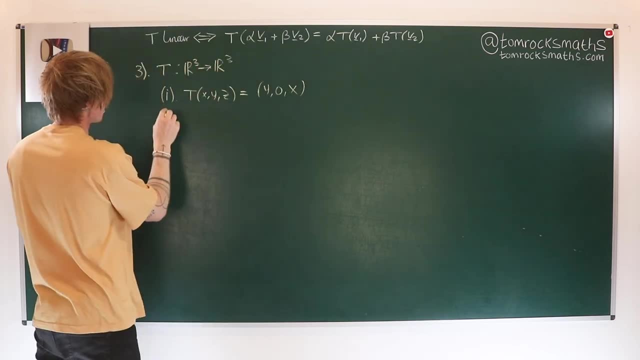 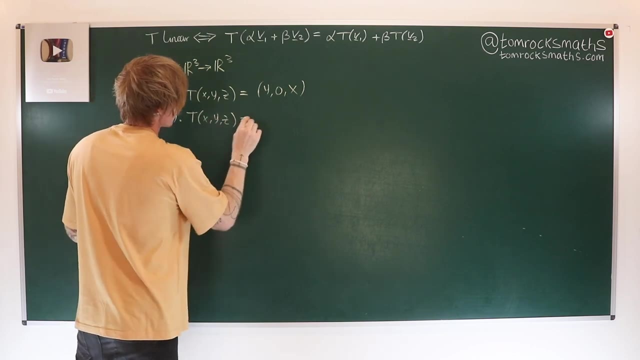 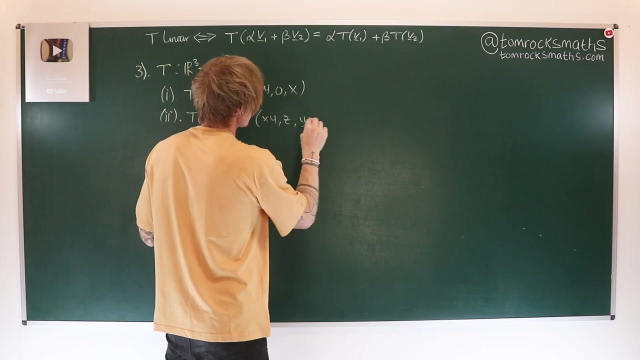 input a general point- x, y, z- it's going to output y, zero, x. Our second one again: if we input a general point and x, y z, then this one is going to output x, y, z, y, z. and our third one in this: 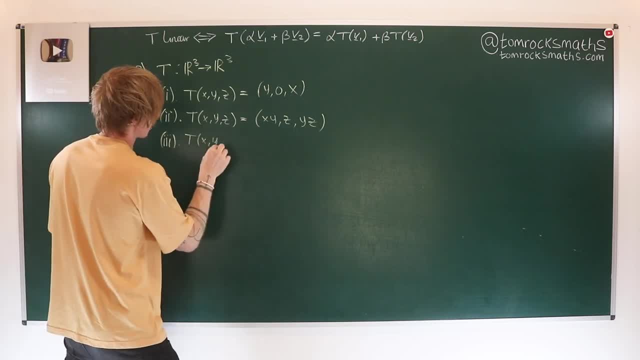 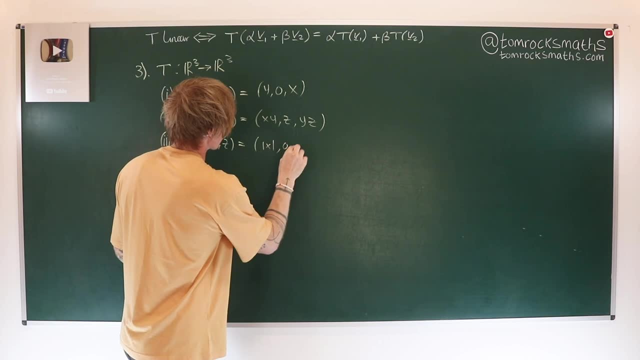 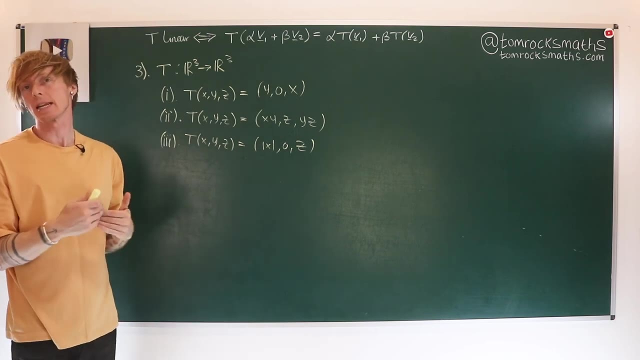 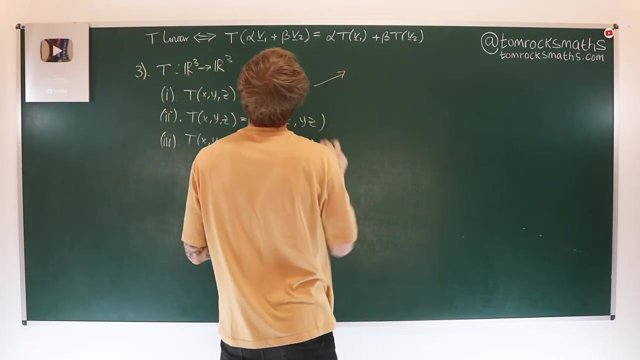 example, again t, general point, x, y, z, but this time let's suppose it gives me modulus of x, 0, and z, and the question is: which of these, if any, define linear transformations? So let's start with the first one. So we want to consider over. 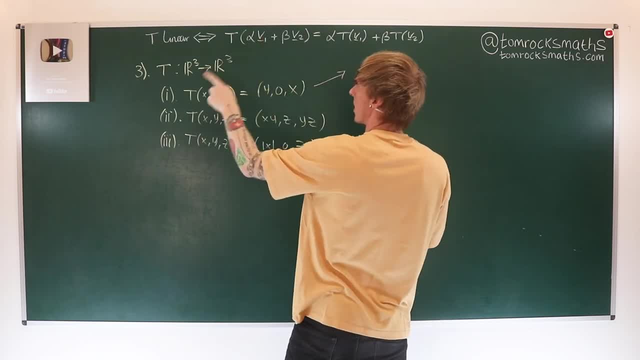 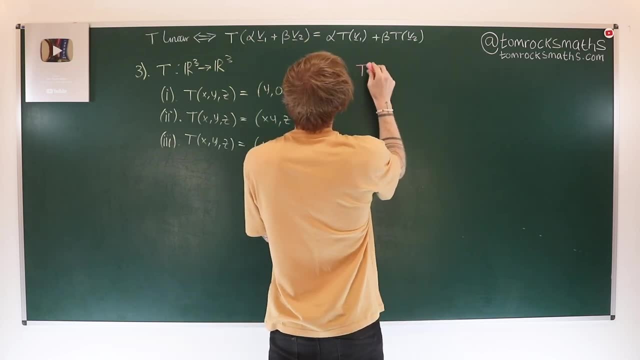 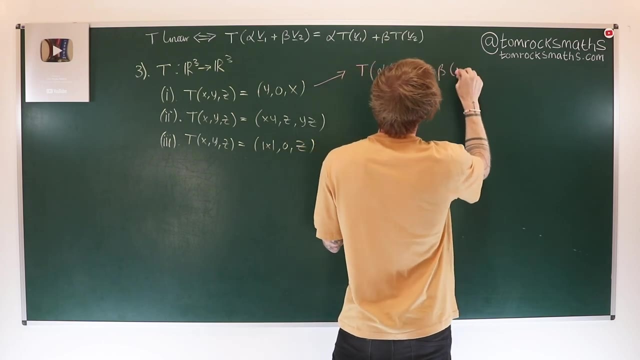 here scalar multiple of one vector plus scalar multiple of a different vector, So that here is going to be t of, let's say it's alpha of x, y, z plus beta of x-hat, y-hat and z-hat. 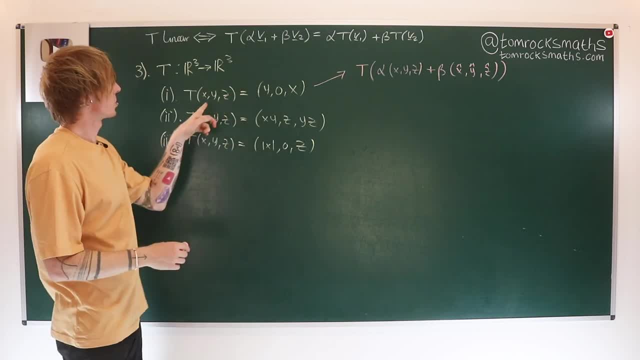 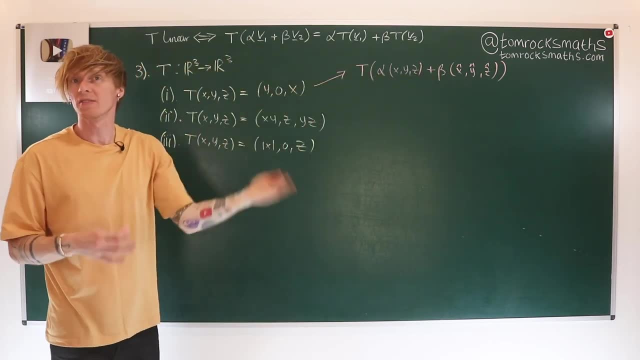 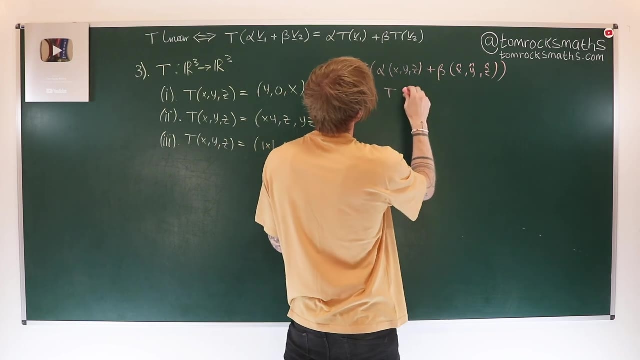 Okay, now we want to apply t to this whole thing and what we've got here is the sum of two three-dimensional vectors. but we know how to add those together, So we can do that inside t. so that's t of the first coordinate is alpha x plus. 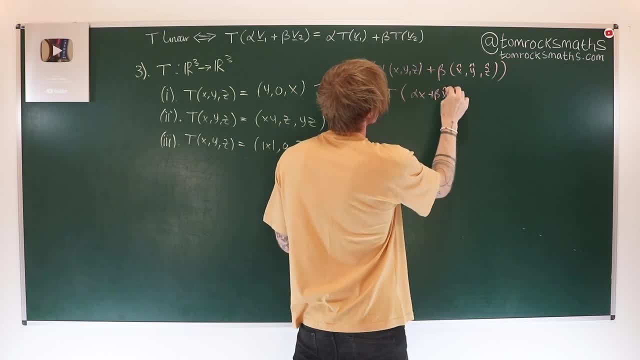 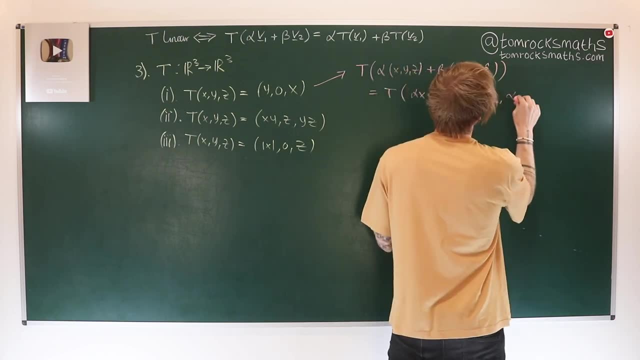 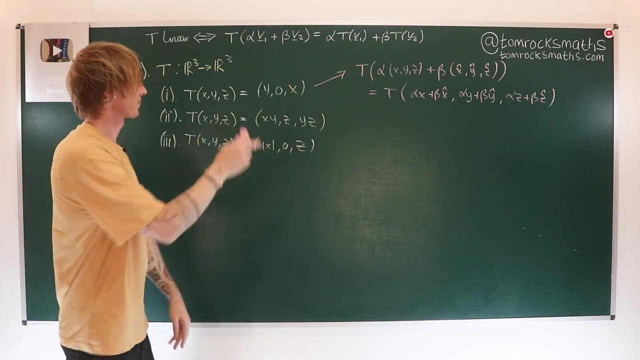 beta x-hat. the second coordinate is alpha y plus beta y-hat and the third coordinate alpha z plus beta z-hat. Now we just have our three coordinate positions and our map tells us: take whatever's in the first place, put it at. 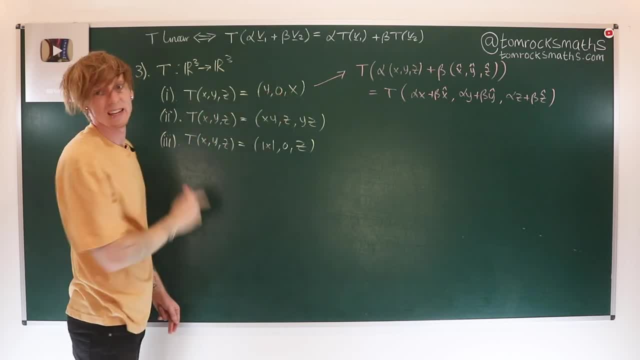 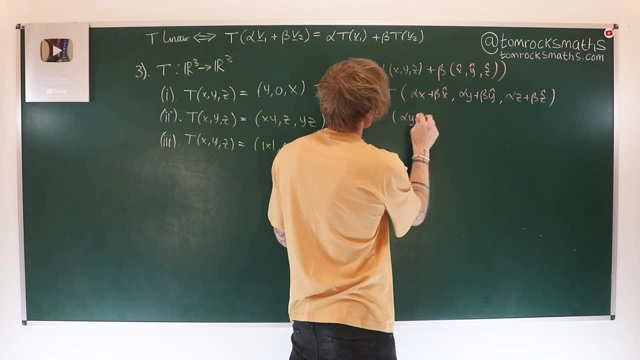 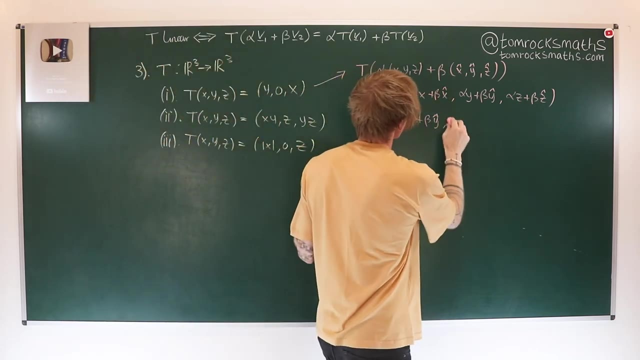 the end. take whatever's in the middle, put it the beginning and a 0 in position 2.. So So this then as an output is going to give me alpha y plus beta y hat. so the thing in the middle has gone to the first position, then a zero, and then I want, I think at the beginning, so alpha x. 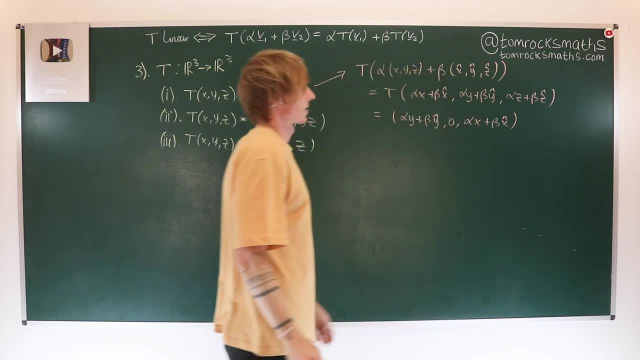 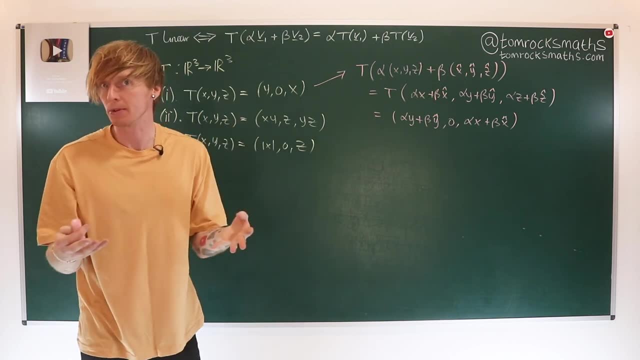 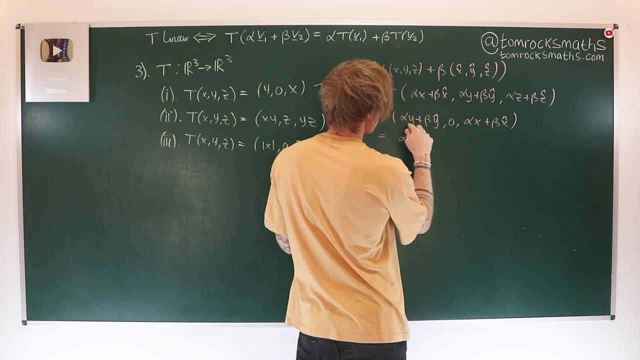 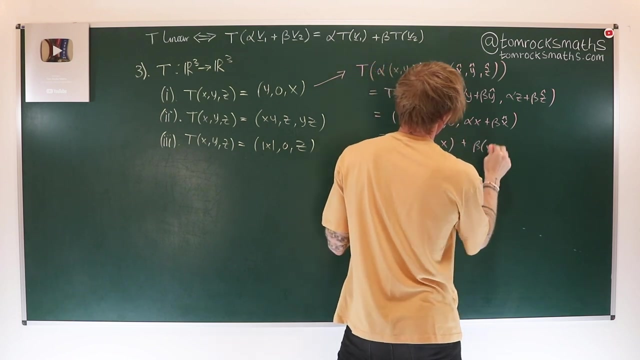 plus beta, x hat. Right now we can split this up again using what we know about adding and the properties, scalar multiples of three-dimensional coordinate vectors. So I can say: well, I've got an alpha times a y, zero x, and then I've also got plus a beta times a y hat, zero, x hat. 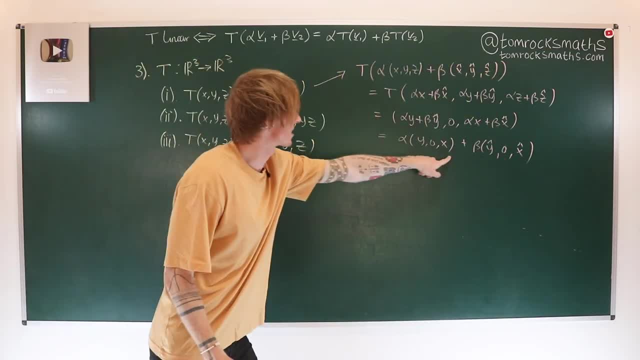 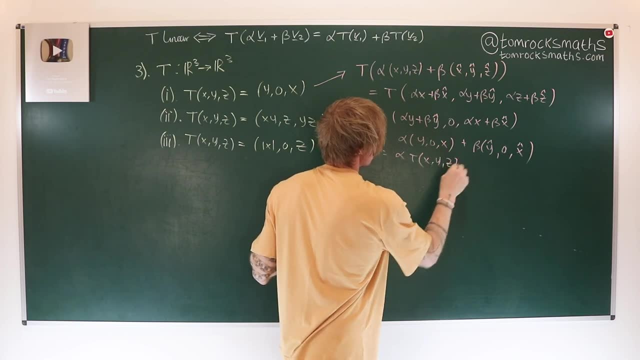 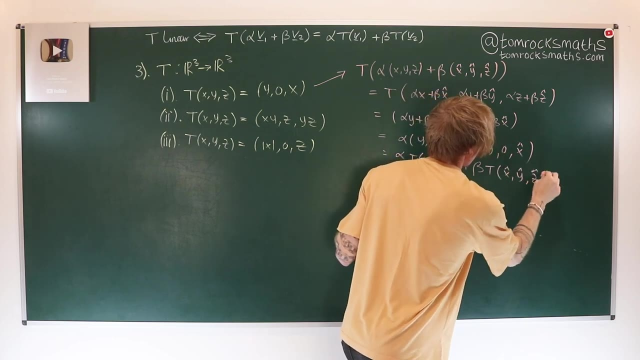 But this looks promising because this is exactly t of x y z. This is alpha times t of x y z, And this one is beta of t x, hat y, hat z hat, So tick. This satisfies the relationship at the top of. 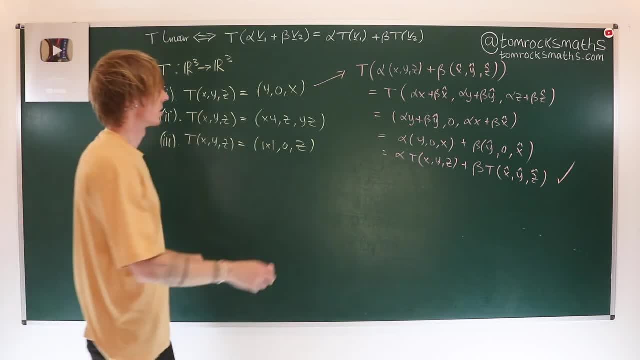 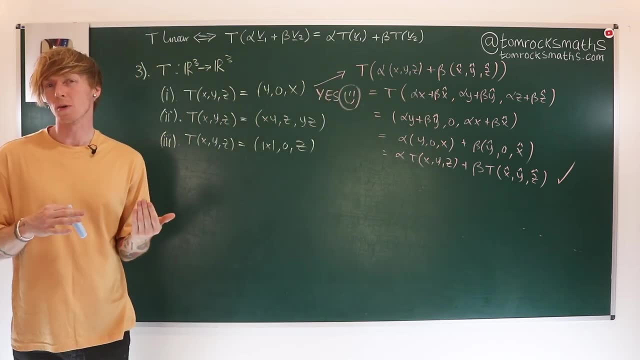 the board. so we can conclude: this is indeed a linear transformation. So this is a big old yes, smiley face. Now for the second one. just by looking at the way that this is defined, it feels like it's probably more. 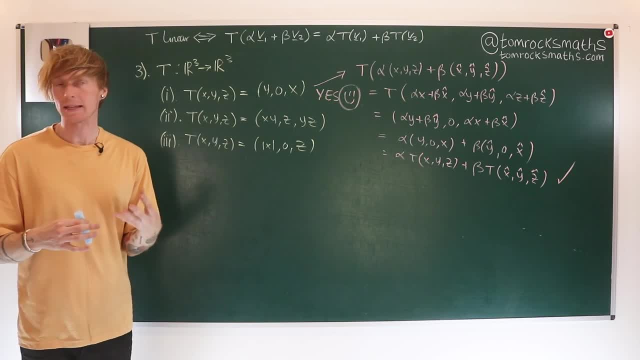 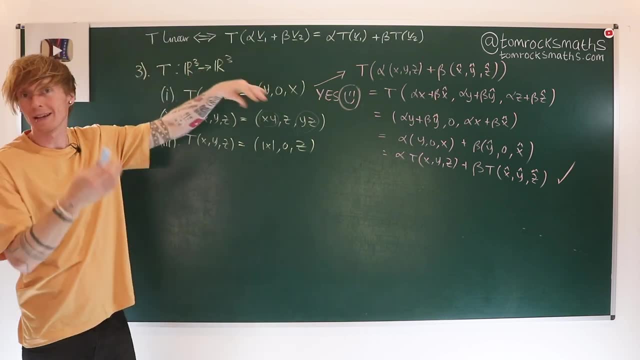 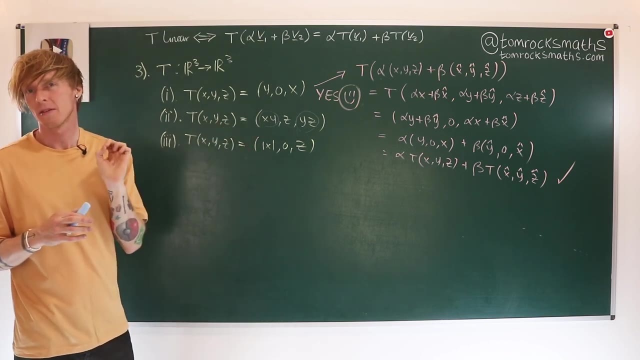 not going to be linear, And the reason I'm saying this is we have these two terms here, which are quadratic. They are two values multiplied together. So this feels like doesn't prove anything, but it feels like it might fail. So what I'm going to do first is check. 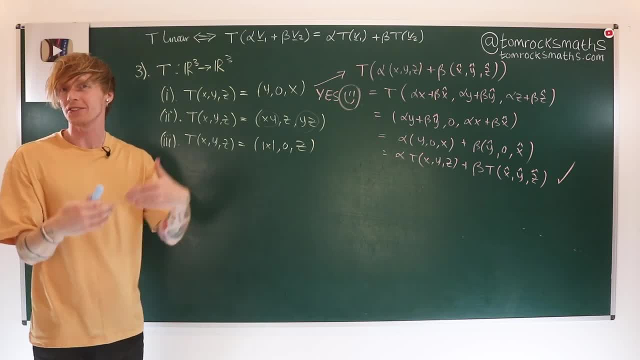 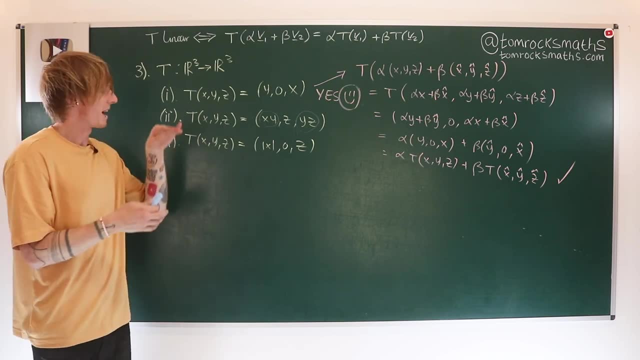 the zero condition, because we know that if it fails the zero condition, it's definitely not a linear map. Of course, if it satisfies it, I'm going to have to do more work, But it feels like it won't be, so I'm going to start by looking at zero. 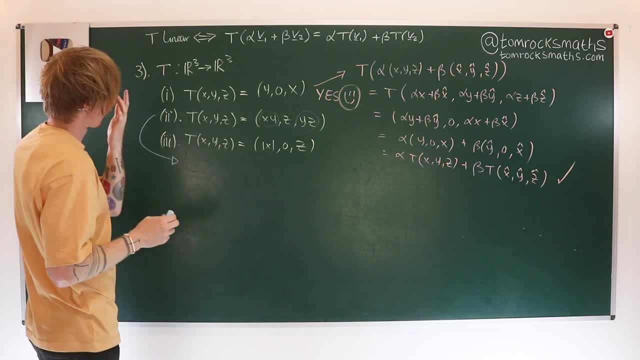 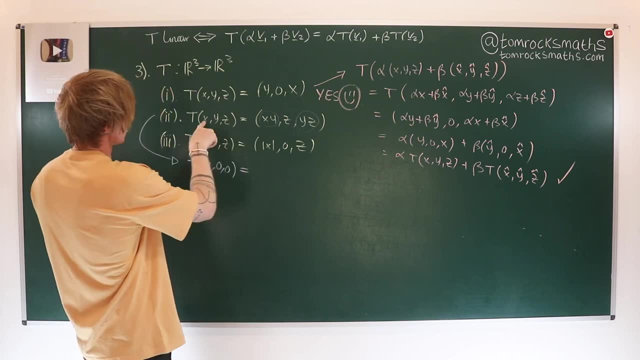 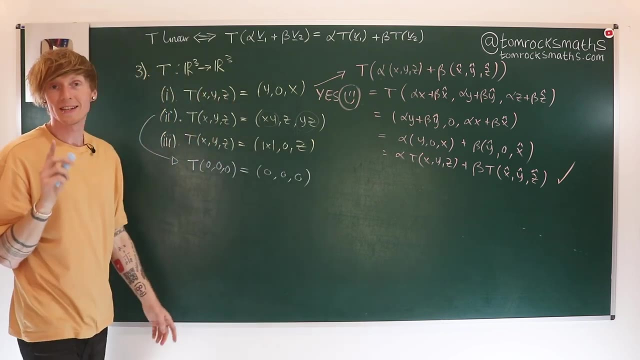 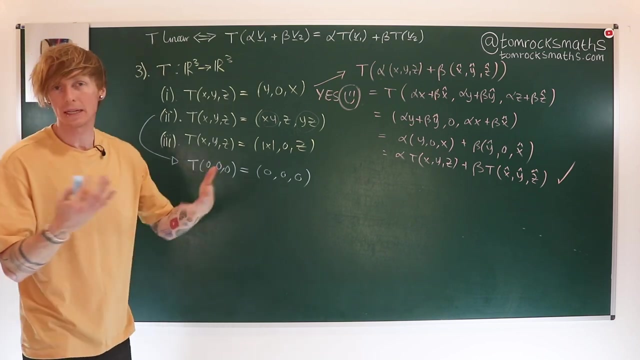 So I do this one down here. So we consider zero, Then t of zero, zero. zero is first two, so that's definitely a zero. Z becomes zero. Okay, so it does satisfy zero. So again, that does not prove it's a linear map, but I can't immediately rule it out. 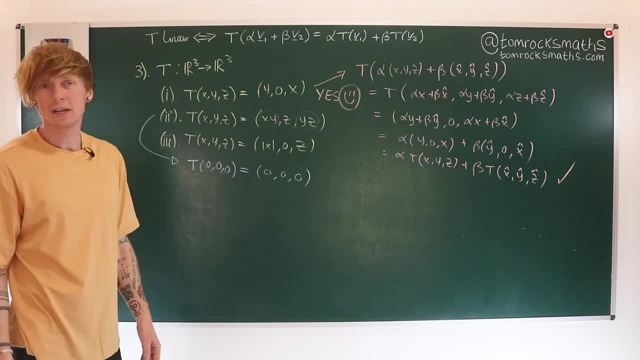 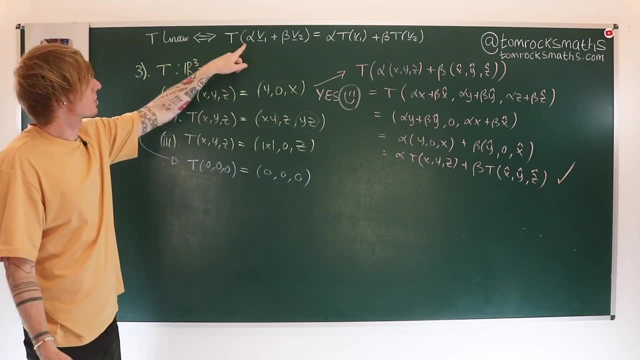 So I'm probably going to have to try using the actual definition. But what I'm going to do here- and this is another helpful sort of shortcut when you think it's going to fail- is I'm going to make alpha and beta one. Both of them are going to be one. 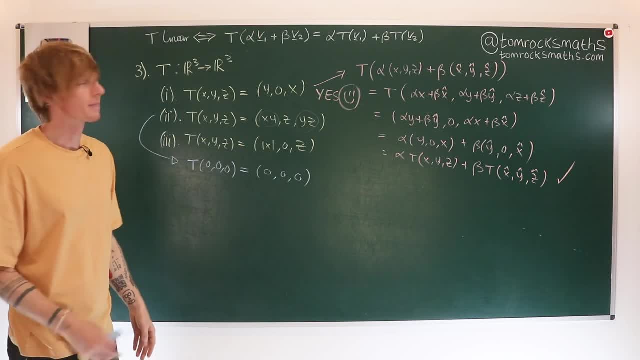 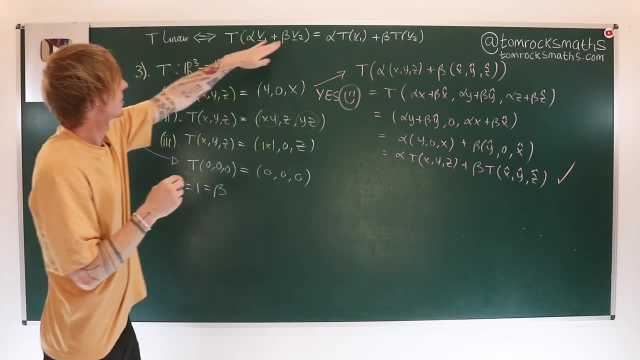 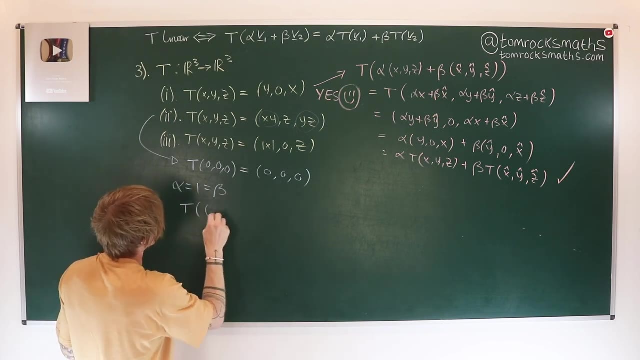 just to simplify a little bit the algebra that's happening. So if I consider alpha equals one, equals beta, and now I want to look at v1 plus v2.. So I want to do as I had it right in red t of it's now going to be x, y, z plus x hat, y hat, z, hat. And again, I've just simplified this. 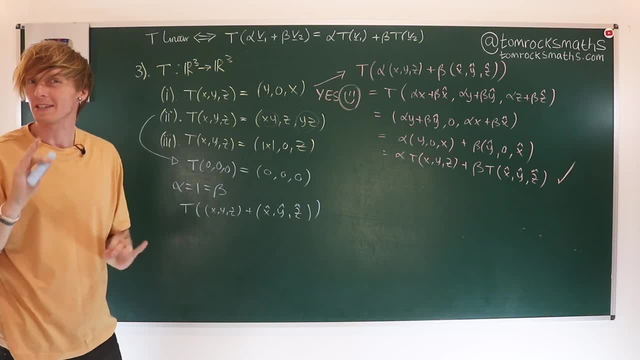 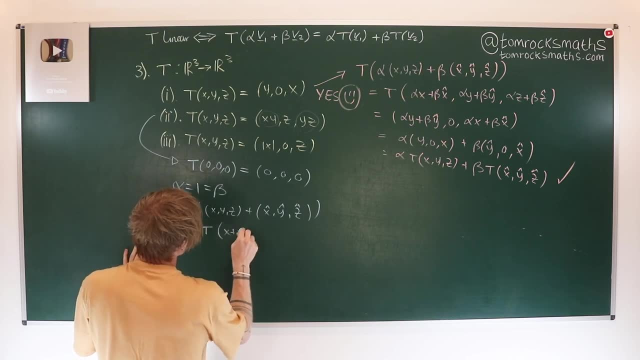 by making alpha and beta both one, because I'm pretty sure it is going to fail, So we can add these two bits together just like we did before. This is t of x plus x hat, y plus y hat and z plus z hat. Now we've got our three coordinates, So this tells us. 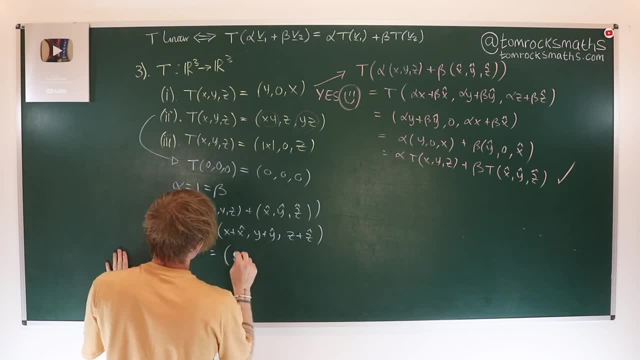 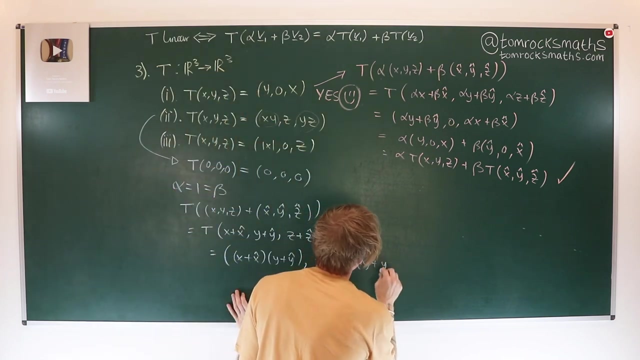 to multiply the first two together. so the output here is x plus x hat times y plus y hat in the first position. The second position is just the third coordinate, so that's now z plus z hat, And the last position is y times z, so that's the second one times the third one, So y plus y hat. 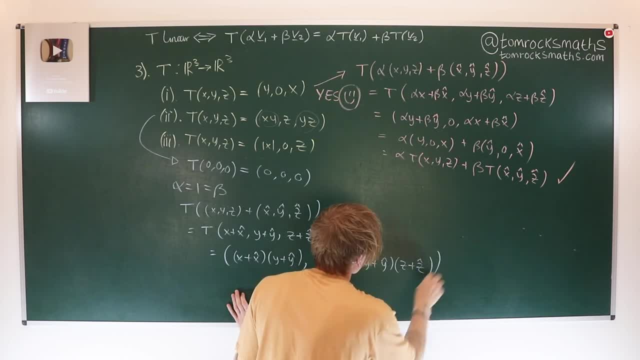 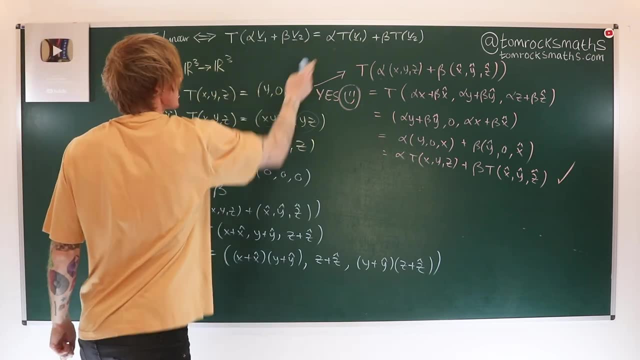 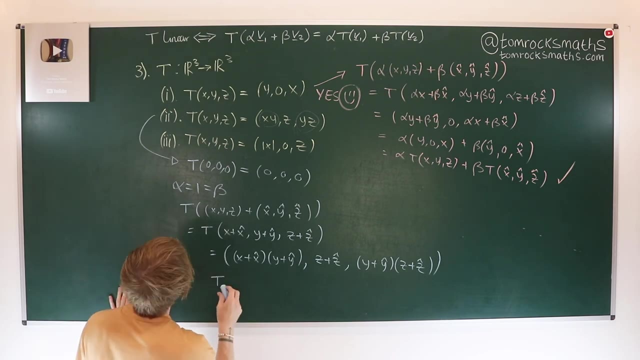 multiplied by z, z hat. Okay, so this is my output Now, if I consider the right hand side up here. so if I say, while that is going to be t of x, y, z plus, because again alpha and beta are one, 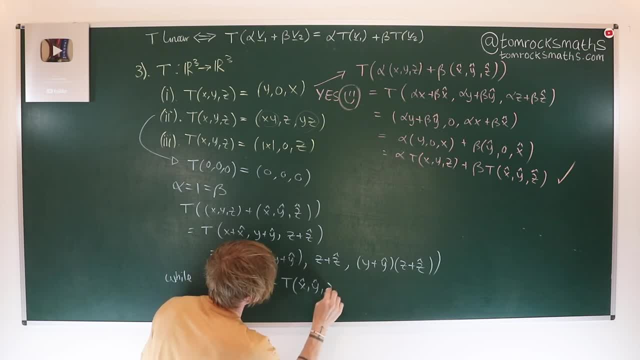 plus t of x hat y hat z hat. Then I can say: well, that is equal to x y z plus x hat y hat z hat. So I can say: well, that is equal to x y z plus x hat y hat z hat, y hat z hat. 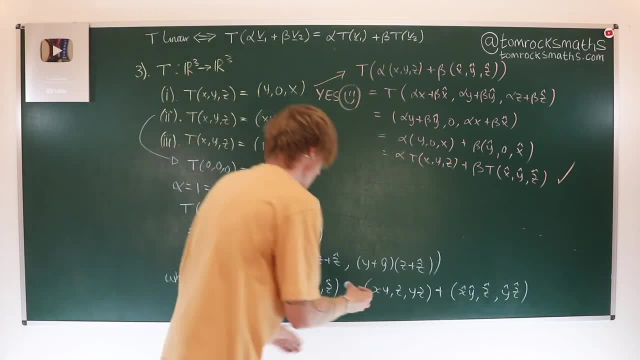 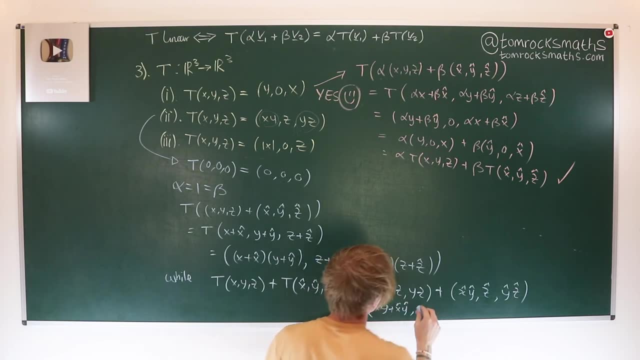 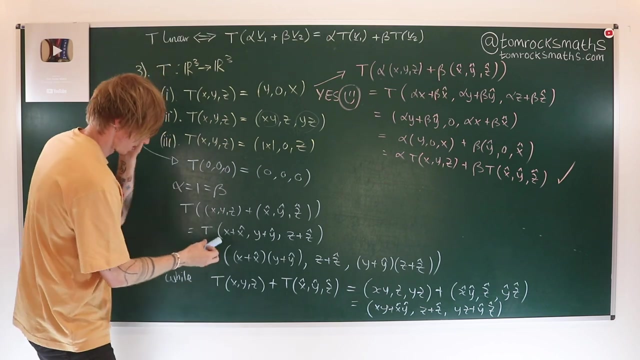 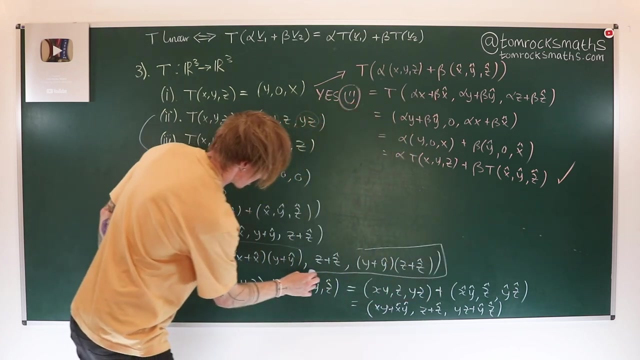 So again, I can add these together. We know how to add together vectors And that's going to give me x y plus x hat, y hat, comma z plus z hat, comma y z plus y hat, And this is not the same as what I've got here. So this in the box needs to be compared with. 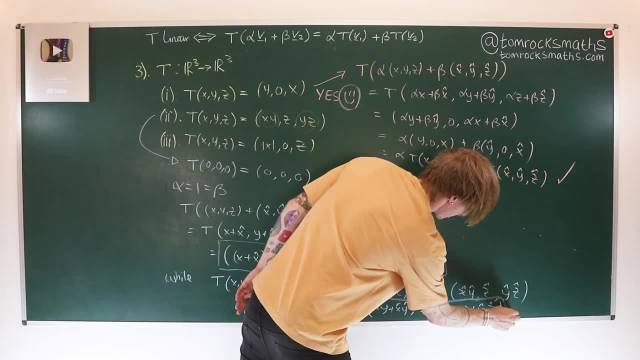 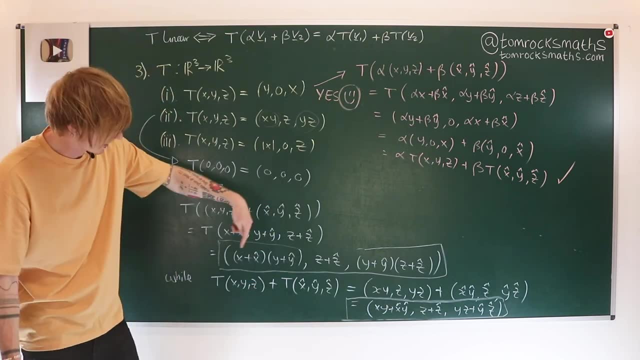 the one in the box down here And with a little bit of thought you can see they're not going to be the same. So if I were to expand out these brackets, I would get x, y. I'd get an x hat, y hat. 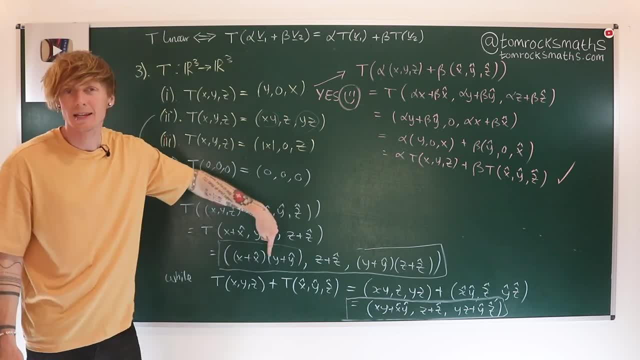 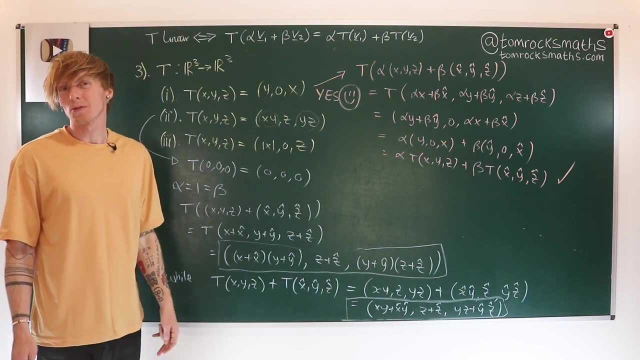 but I'd also get an x y hat and an x hat y, So I'd get a cross term when I expanded out these brackets And down here. we do not have cross terms in those first or third positions. So the second position works. We have z plus z hat, and here we also have z plus z hat. 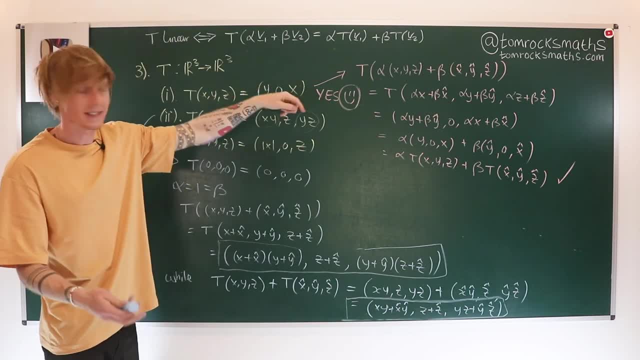 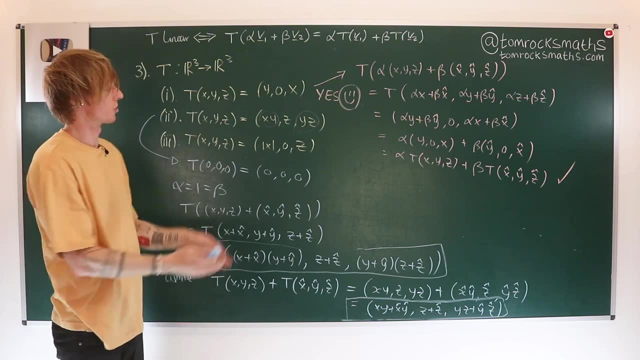 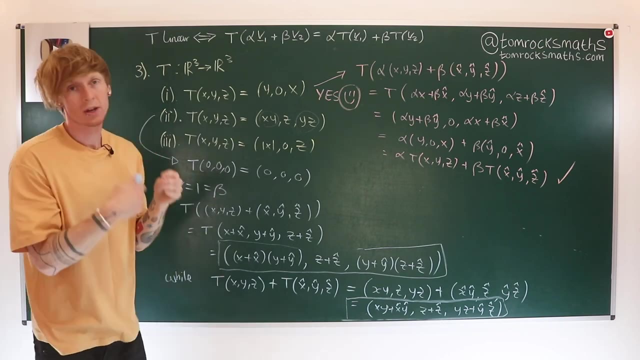 And that's because up here this is a linear term, It's a single power. There aren't several things multiplied together. But these two both fail and of course we need all of it to work, and it has to work for any alpha and beta. So the fact that it's failed when alpha and beta are both 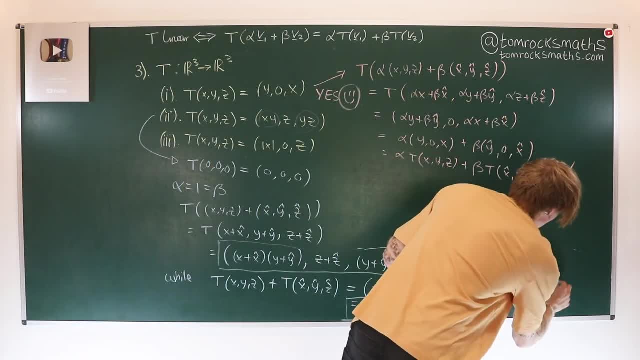 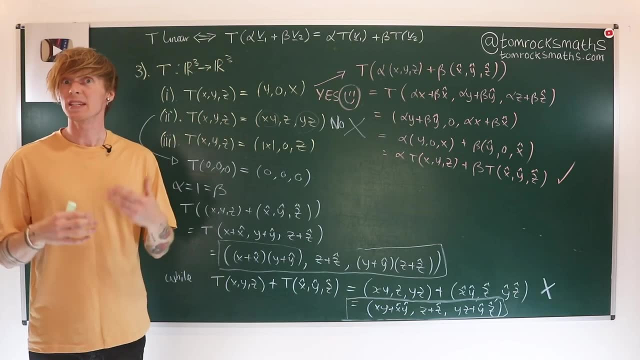 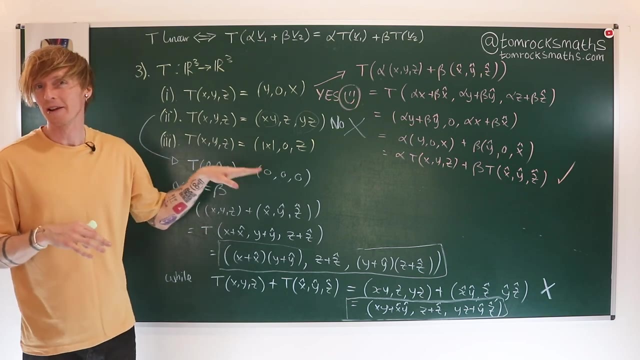 one means this is not a linear transformation. So this one is, no, not a linear map. Now for this third one. I'm going to take another, different approach, but it's sort of related to what I tried to do in the second one, which is to look at what happens around zero. So the modulus. 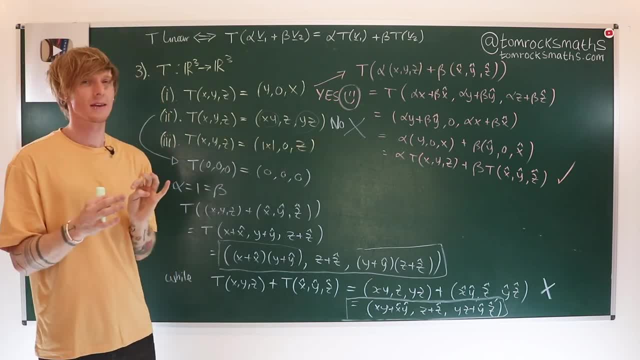 here, I think, is going to be the same as what I did in the first one, which is to look at what happens around zero. So the modulus here, I think, is going to be the same as what I did in the second one. cause problems when we add together positive and negative numbers. that should cancel out. 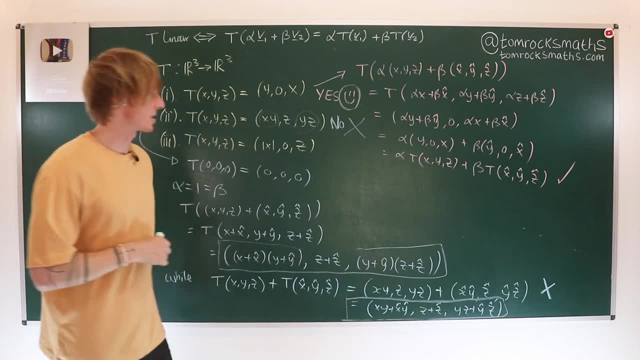 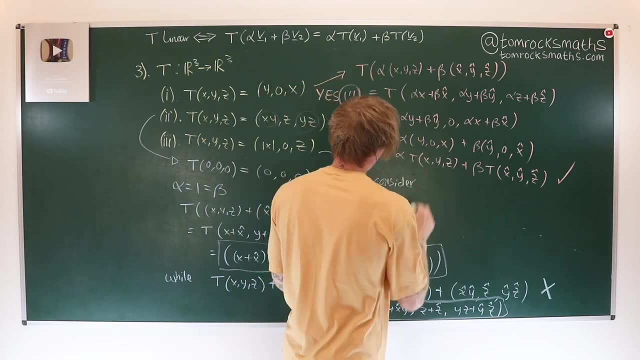 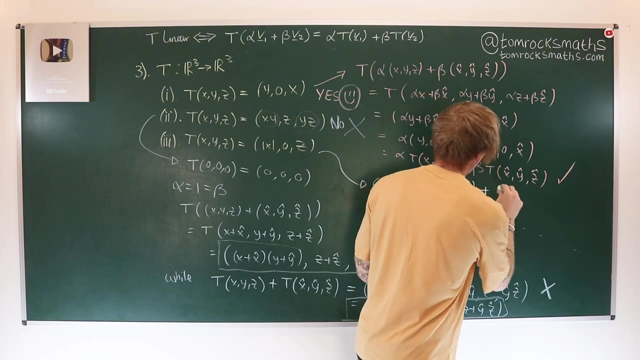 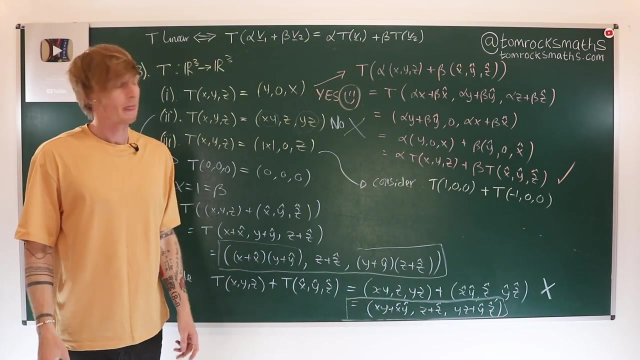 but possibly won't because of the modulus. So here's what I mean If we do this over here. so if I consider two separate inputs, so if I consider t of 1, 0, 0, and I add it to t of minus 1, 0, 0. 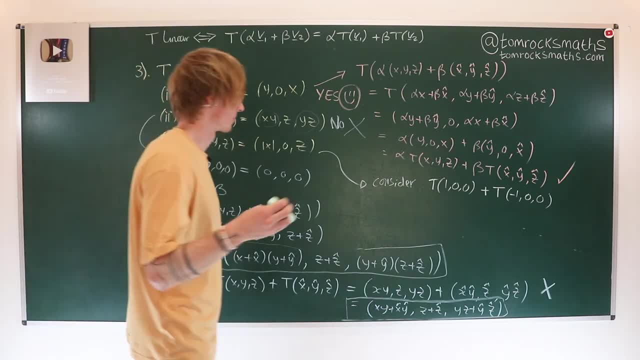 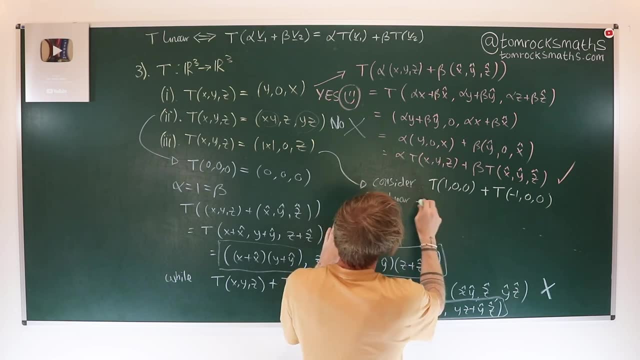 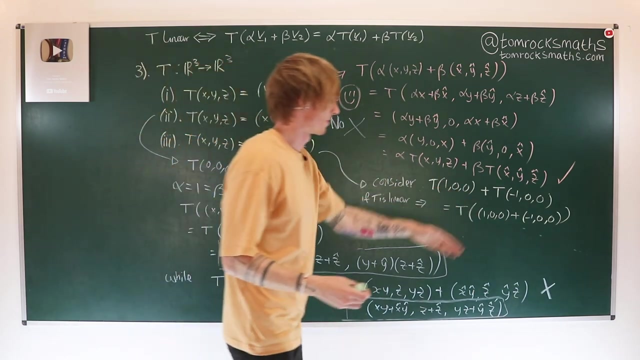 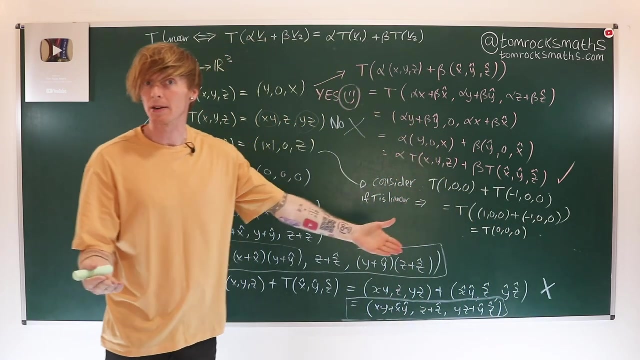 So if t is linear, then this is equal to t of the two pieces added together inside it, like so. But of course when I add them this gives me t of 0, 0, 0. And we know this has to be zero. but I can even check using the definition. 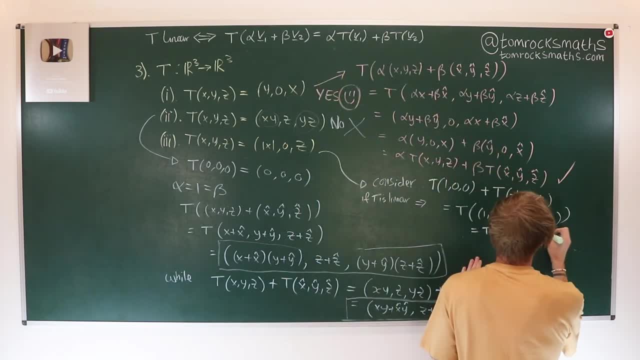 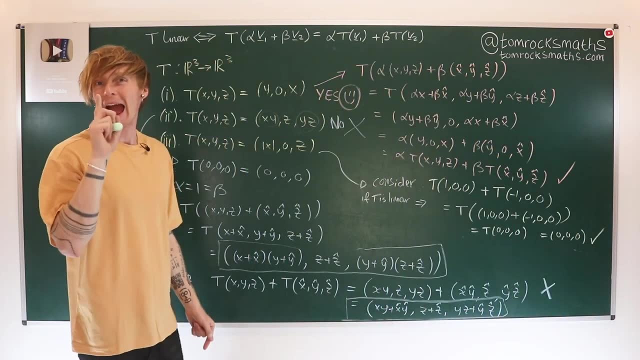 I'm going to get 0, 0, 0.. So this does give me 0, 0, 0, as it has to if it's going to be a linear transformation. However, this was using linearity, so we brought. 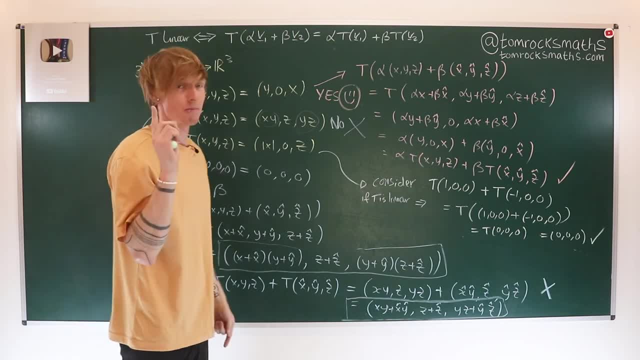 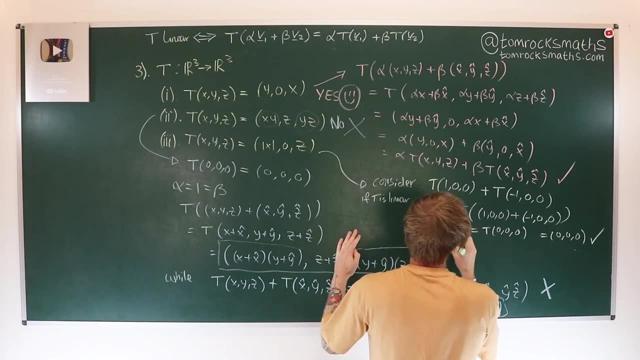 them inside t, so we assumed it was linear. But the problem is if we look at these pieces individually so we can say: but t of 1, 0, 0 is 1, 0, 0, and t of minus 1, 0, 0 is 1, 0, 0, because of that modulus. 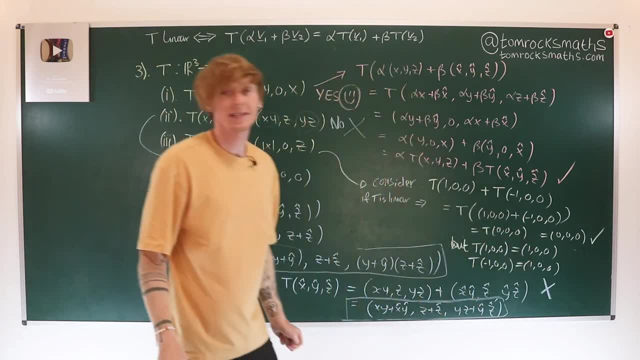 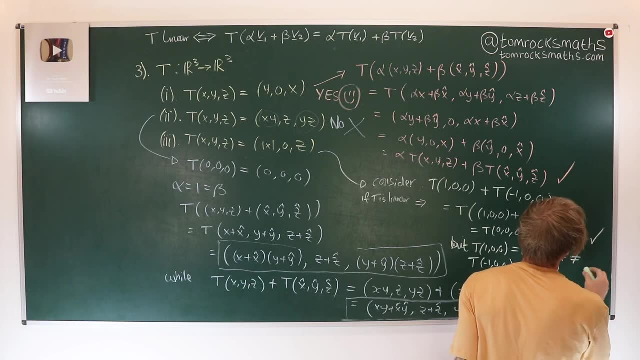 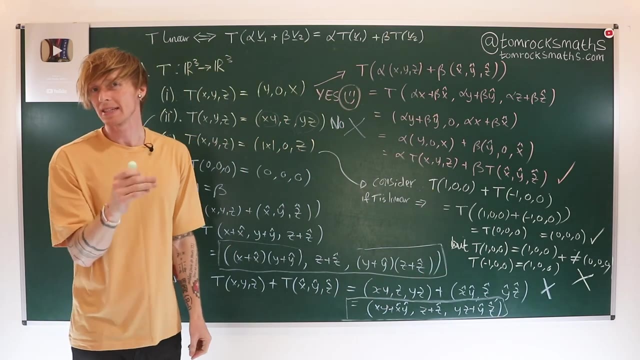 on the x. So when we do them individually we get these two pieces, And now if I add them together in the final subspace- w add them together- we do not get t of 1, 0, 0.. 0, 0, 0. So it actually is going to fail on that zero condition. 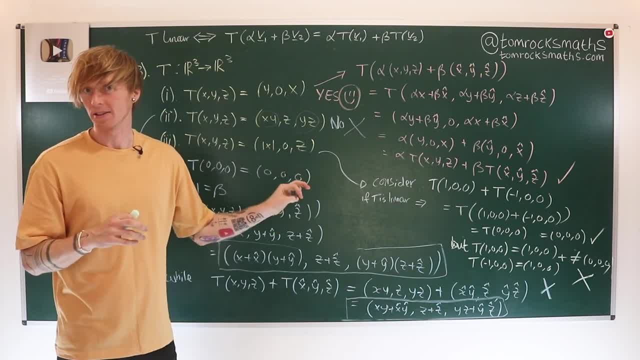 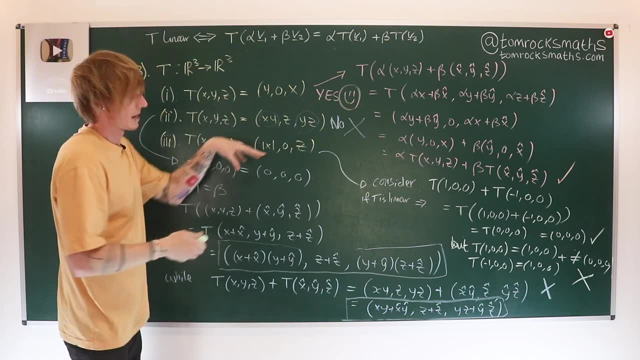 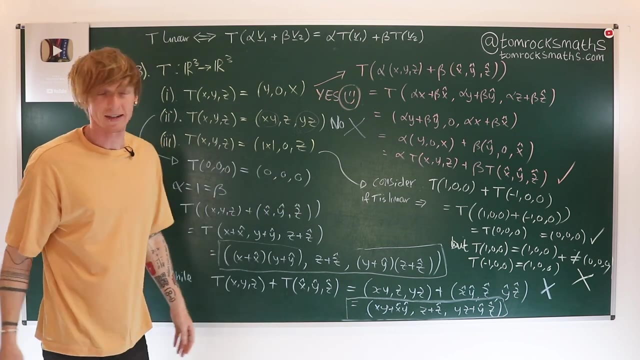 So it is important to note how this actually failed. It wasn't a case, like I did in the second one, of inputting 0, 0, 0 and checking it outputs three zeros. So sometimes that will work: you'll input three zeros and it will not give you the zero vector. But here it does right. We input: 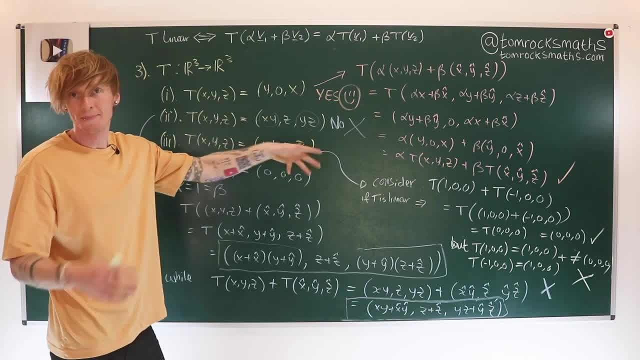 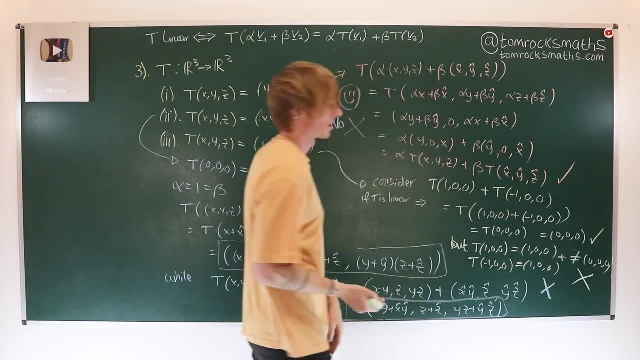 0, 0, 0, we get mod of 0, 0, 0 and 0 again. So that's fine. But what we can do is we can construct two pieces cleverly like this: It can be any number with opposite signs. in fact, in the x 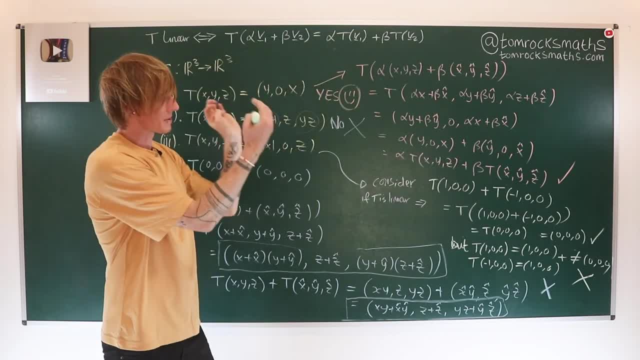 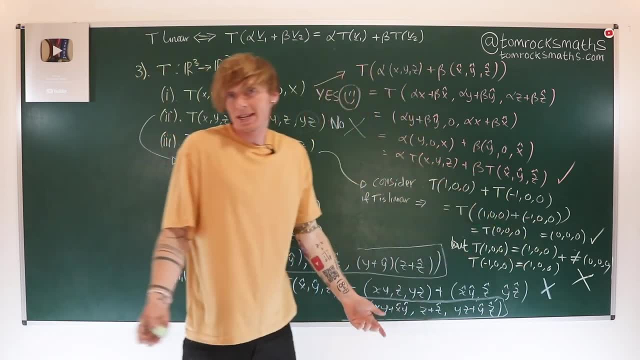 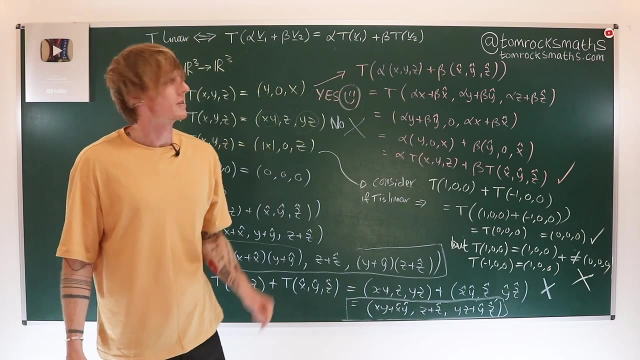 position, And then we can add them together inside t, assuming it is linear, and that will give us zero. It has to give us zero, But if we treat those pieces separately, we don't get zero. So what it's doing is it's failing this. We've found a particular 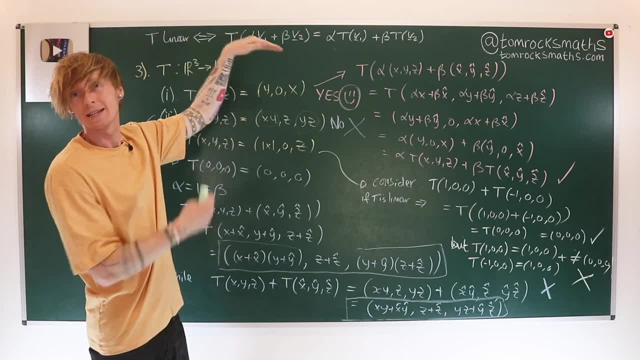 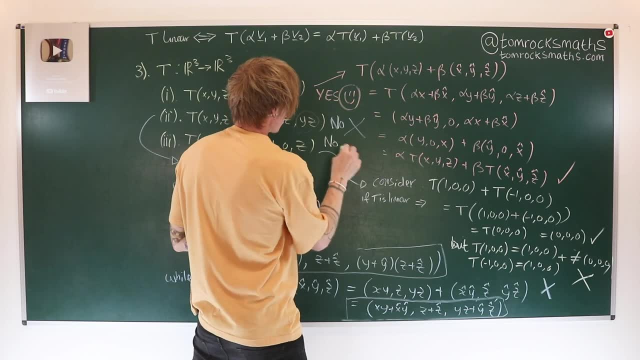 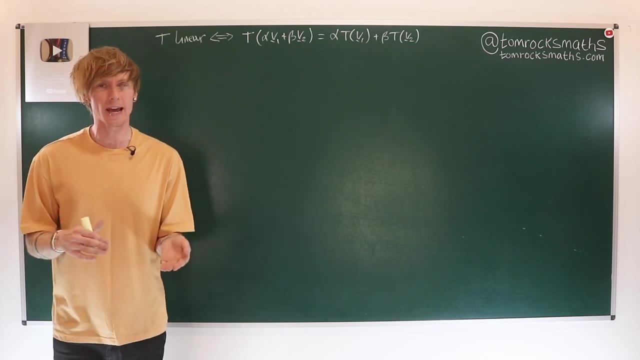 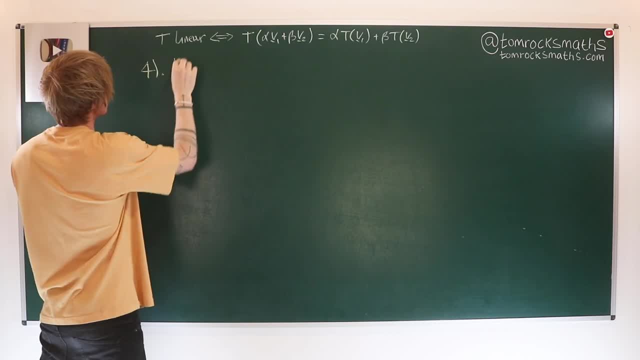 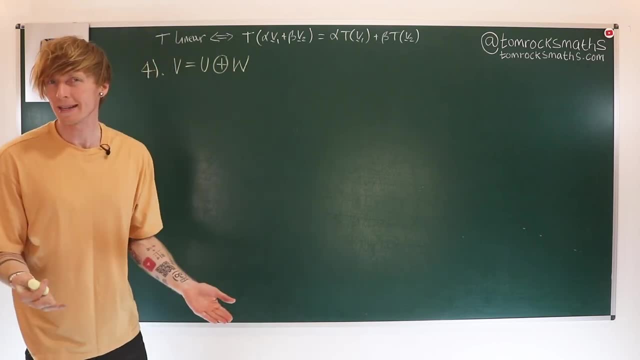 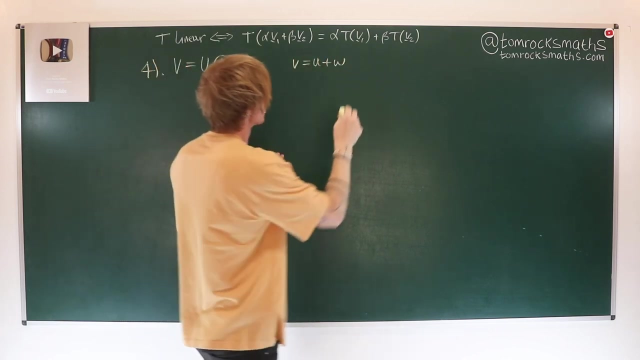 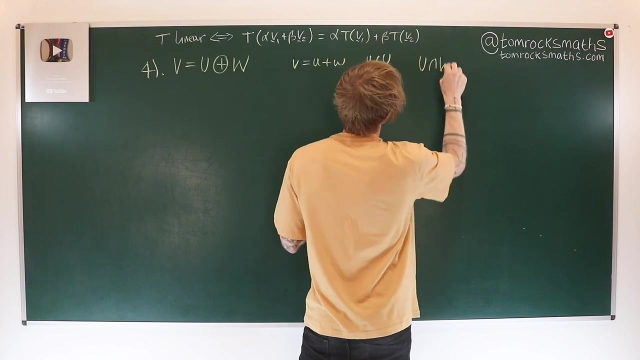 Let's suppose we have a vector space, V, which is equal to the direct sum of u and w And, as a reminder, this means that any vector in the space is written as a sum of two pieces, where u is in u and w is in w, And we also know that the intersection of those two spaces 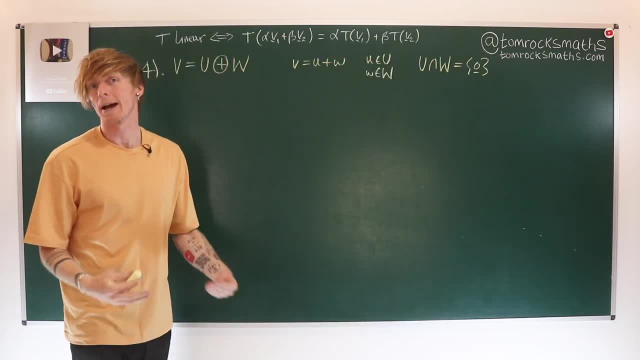 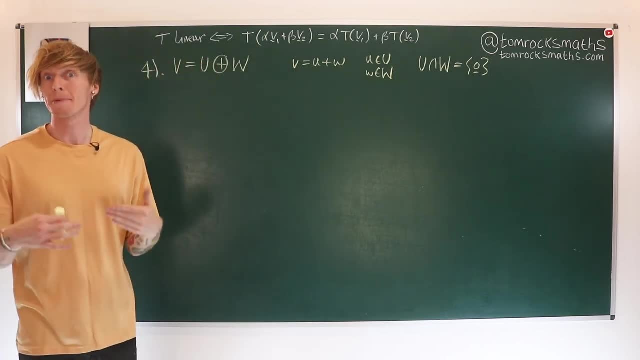 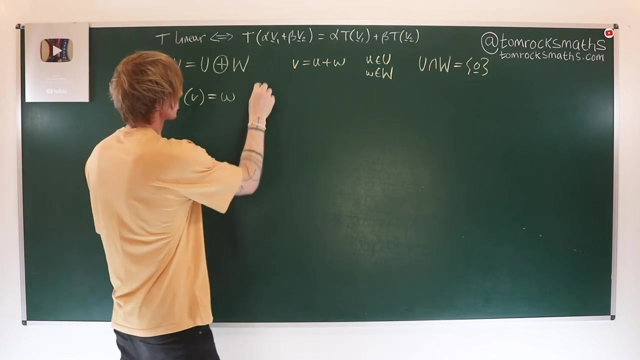 is only the zero vector, so there's no overlap between them apart from zero, which has to be there if they are both true vector spaces. We're going to define a map p as follows: p of a vector, v, is going to be equal to w and this is called. 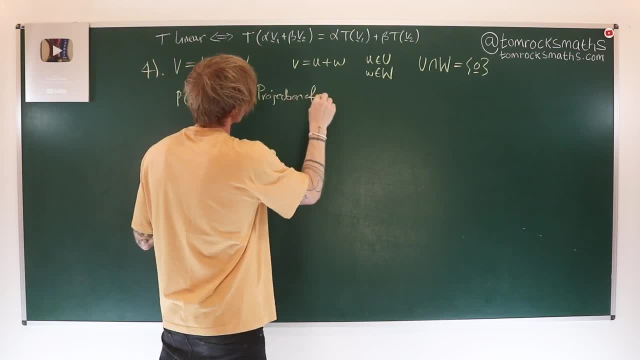 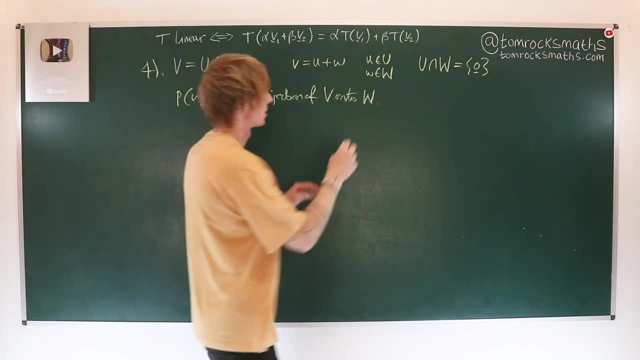 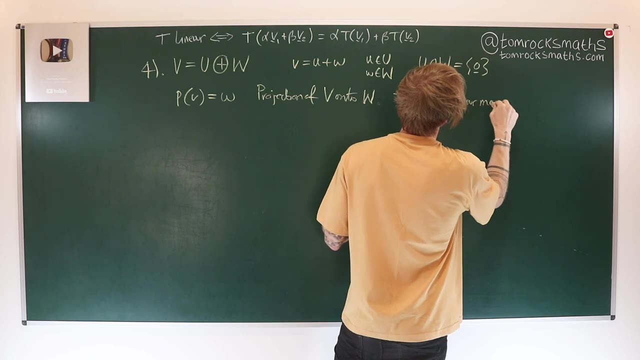 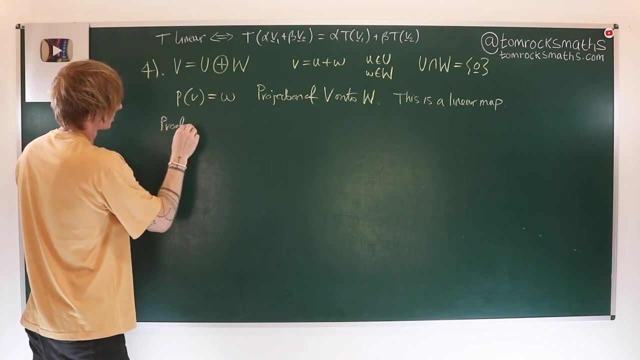 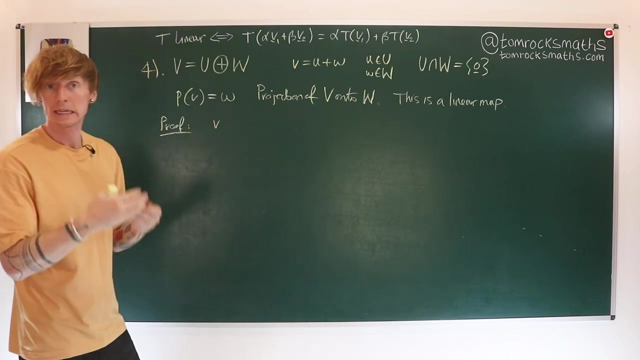 the projection of v onto its subspace w. I'm going to claim this is a linear map. Now, of course, we need to prove this. so proof, We can start by saying: well, we know, for any vector v in our space. 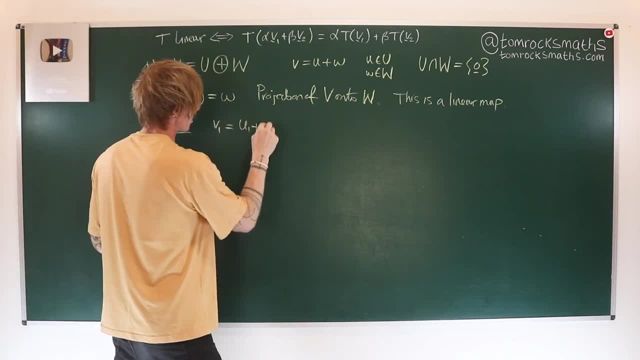 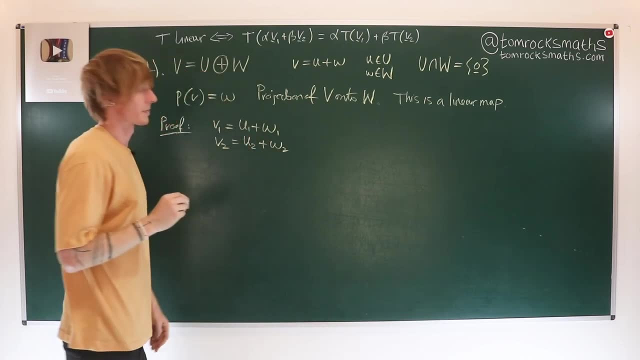 so let's say v1. we know it's equal to u1 plus w1. and if we have a set, we now get to top ainadoice, which will get us to a space vector v2. we know that is u2 plus w2.. So now we know what our two pieces look. 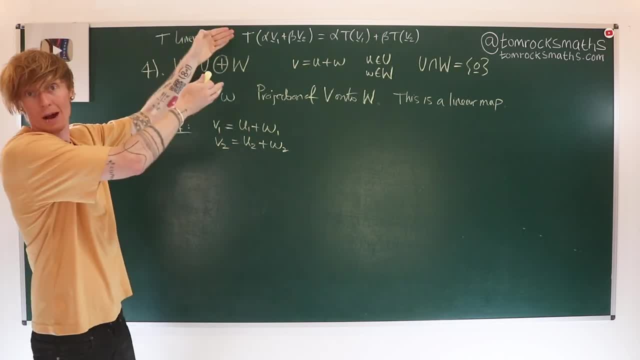 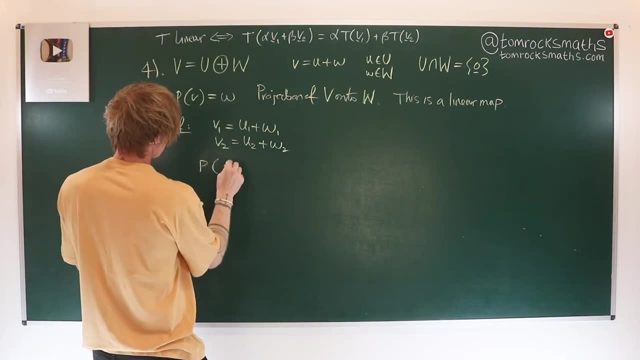 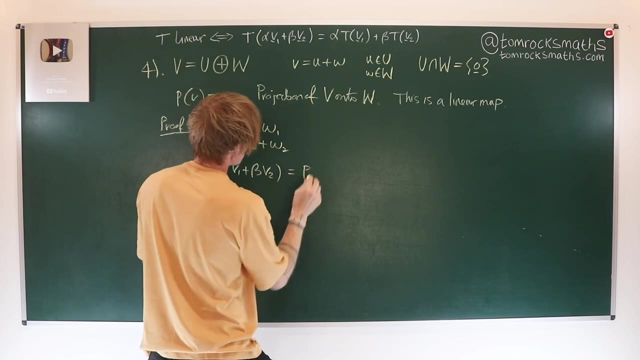 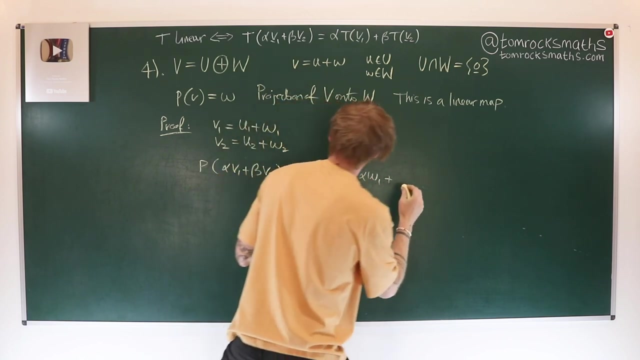 like we can now consider the left-hand side of our condition to be a linear transformation. So if we now consider P of alpha v1 plus beta v2, then that is P of this whole thing. so that's alpha u1 plus alpha w1 plus beta u2 plus beta. 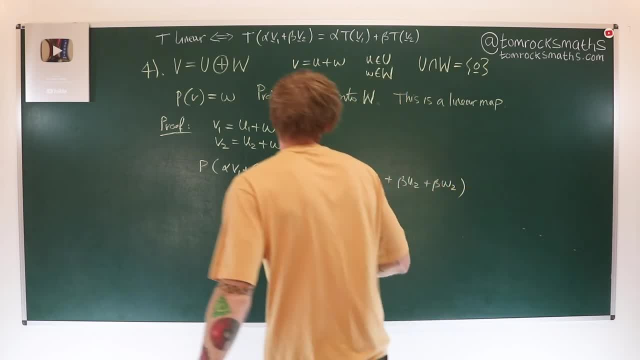 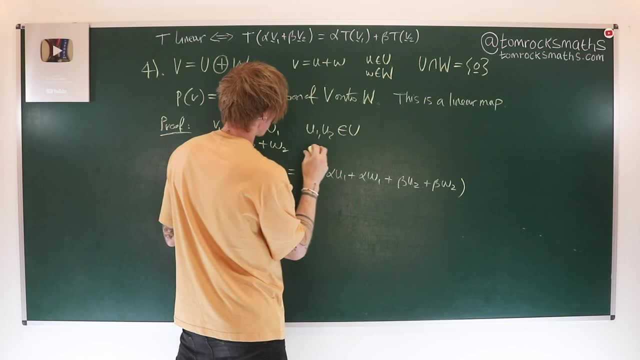 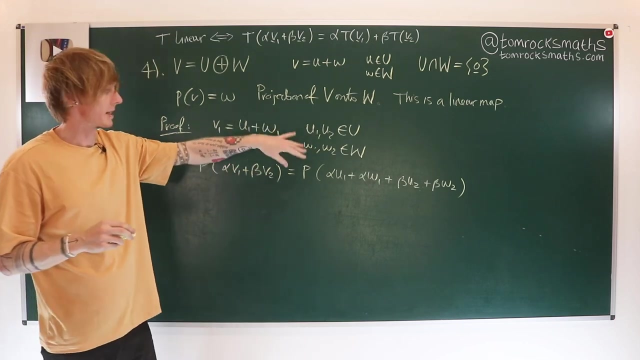 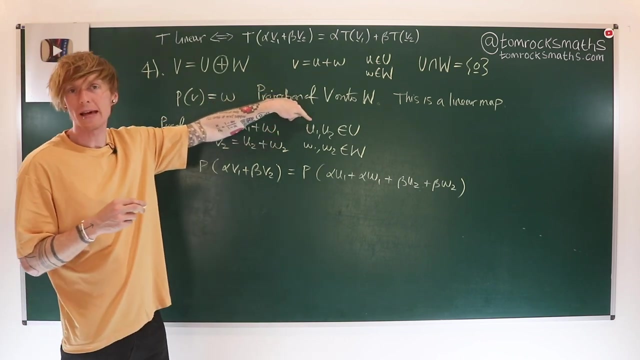 w2.. Now, given that we know u1 and u2 belong to u and w1, w2 belong to w. these are subspaces. That is a key part of the direct sum definition. So what that means is, if we add these two pieces together, we stay in our space u and we can also actually add